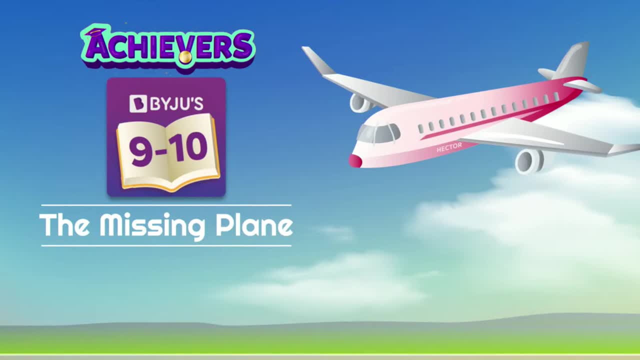 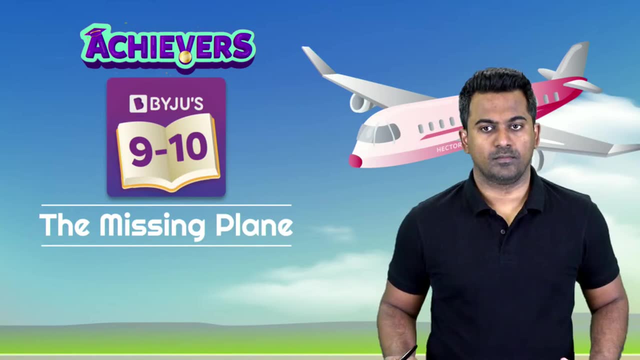 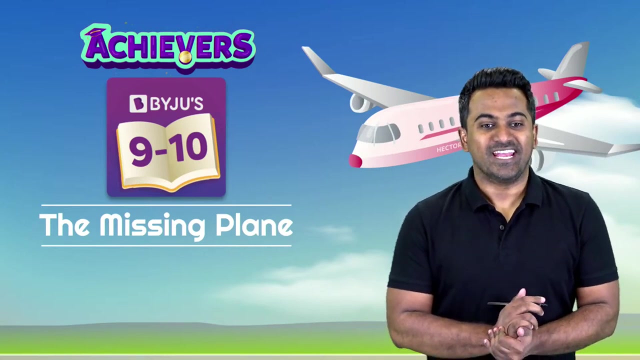 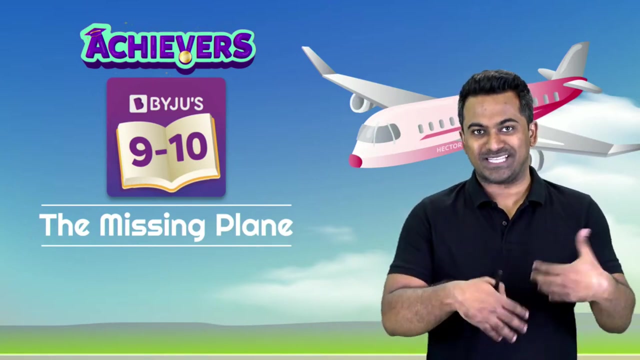 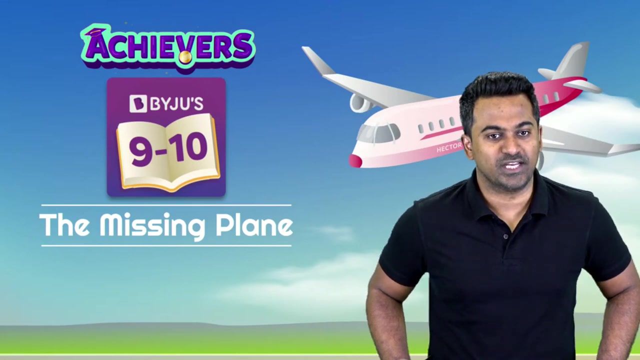 All right, hello everybody, and welcome to the session called the missing plane. Now, this is going to be an introduction to the next chapter, after the topic of number system, whose NCRT we just did. Yes, so we have our students here with us, Tatleen Anushree, we. 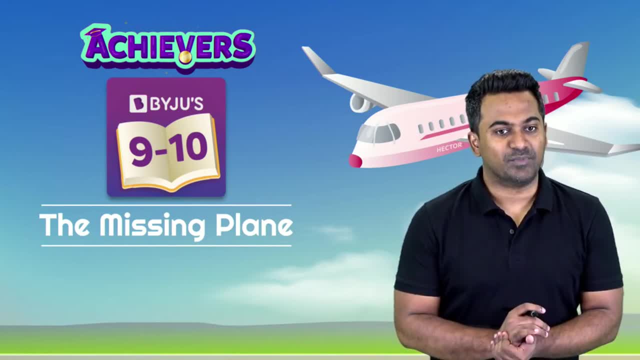 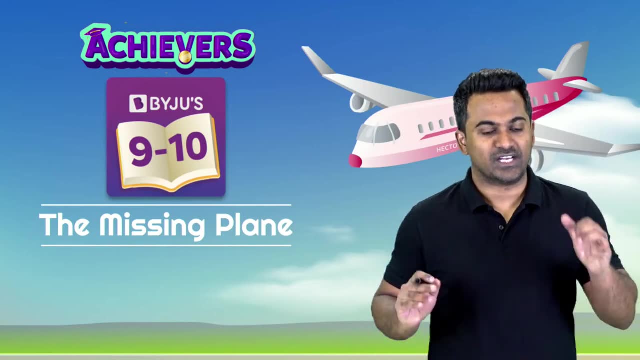 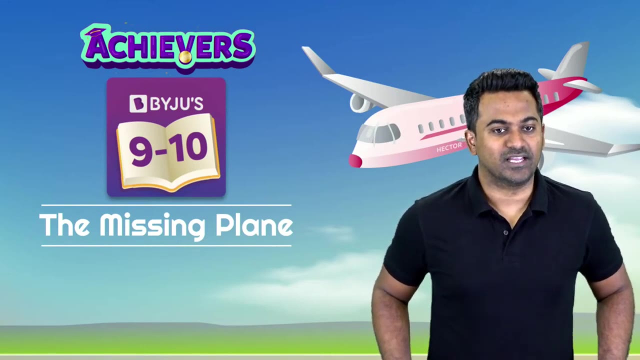 have Madiha. Jyoti Adrika, I believe, has joined us in this session. Yes, Prashansa was there. Divyansh was there. Shafi, hi, Shafi, hey, Muskaan, hello, we have Shivansh. yes, hello Madiha. 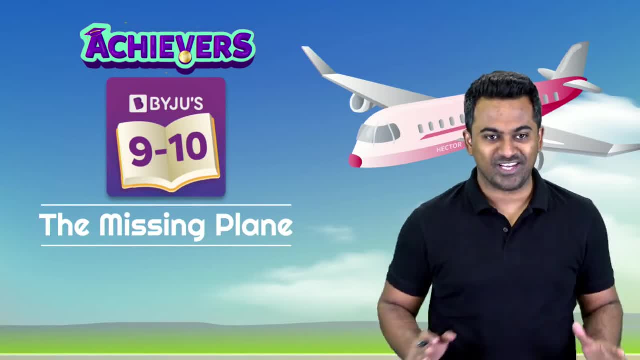 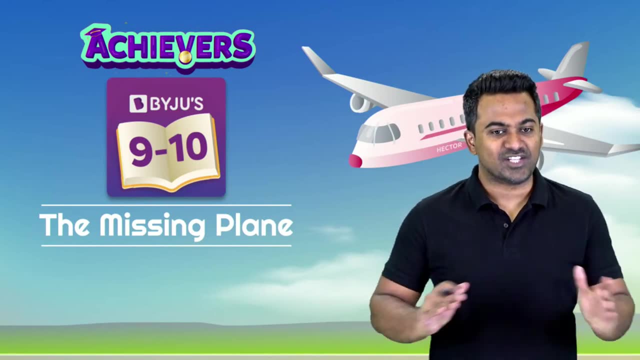 yeah, Rashmi, good evening again. you guys were all part of the session earlier. yes, yes, once again. hello, Prashansa. yeah, Aditi, good evening. hey, Anshal. hi hi Aishwarya. 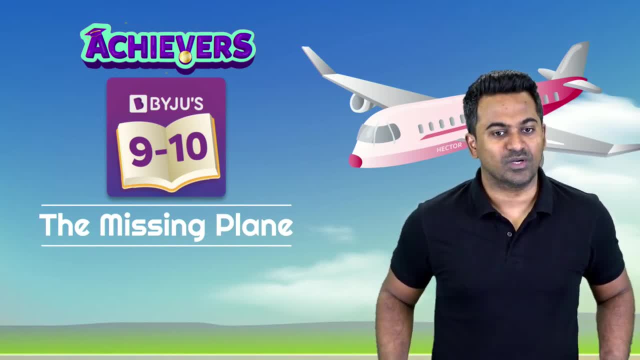 nice to be with you here as well, Anshal. hello hi, Lakshmi again. okay, this time you are early for this session. yeah, cool, so we have Punit Kaur Jyoti Mishra. good evening again, SDT hi. 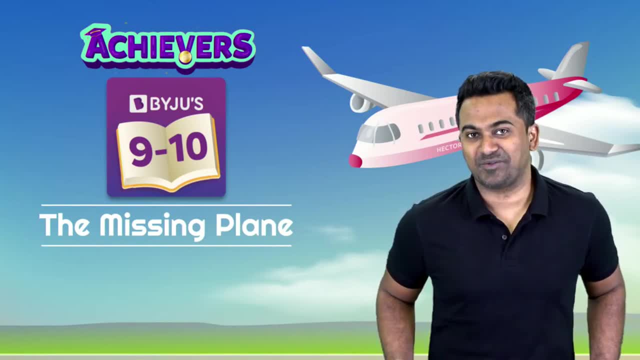 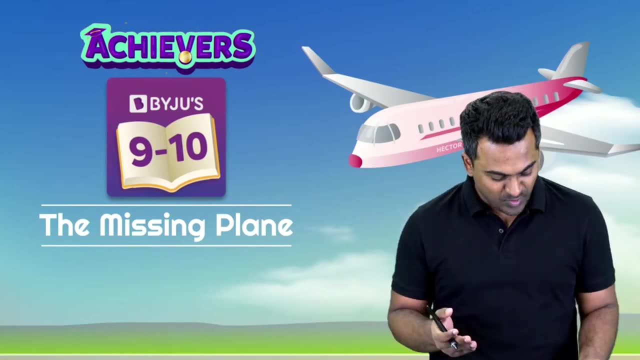 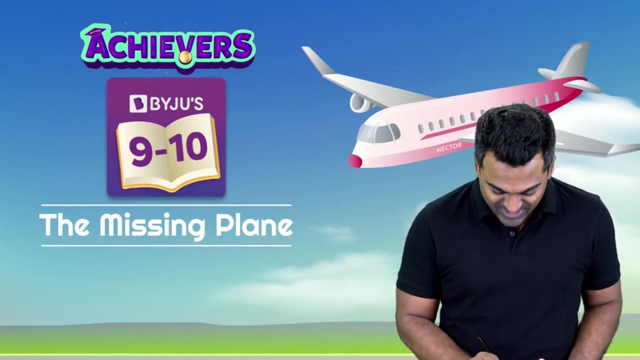 awesome, cool. so are you guys excited about this session? yeah, because, as I said, we're going to a new topic with this session and the name of the topic is going to be the missing plane. so we got quite a lot of stuff to do here in this session, so let's get started. yeah, I hope I'm audible. 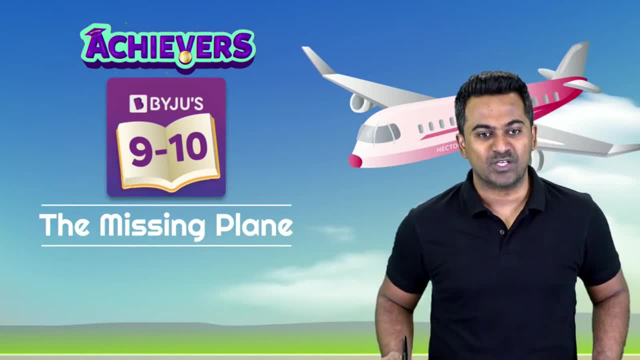 and visible. I, you know, forgot to check that here. so if I'm audible and visible, just quickly give me a thumbs up and then we can proceed. yes, well done the Divyansh Olympiad sessions well. 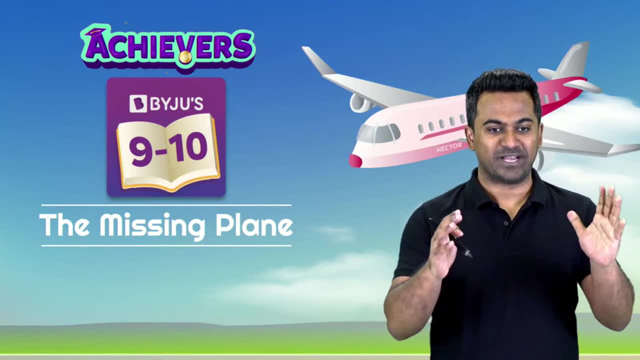 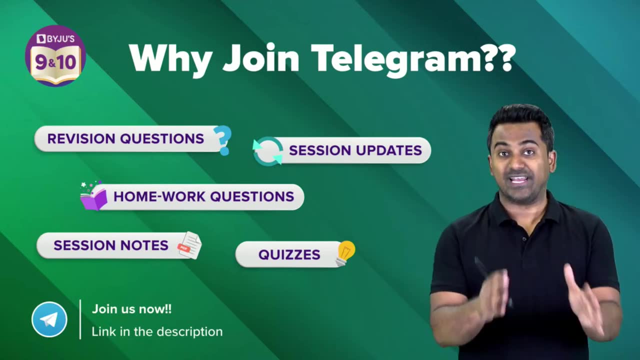 let us know, let us know, we'll let you know that. all right, so I'm getting thumbs up from all your amazing students, so let's begin new students joining us. yeah, I've got to remind you that we have our Telegram channel. 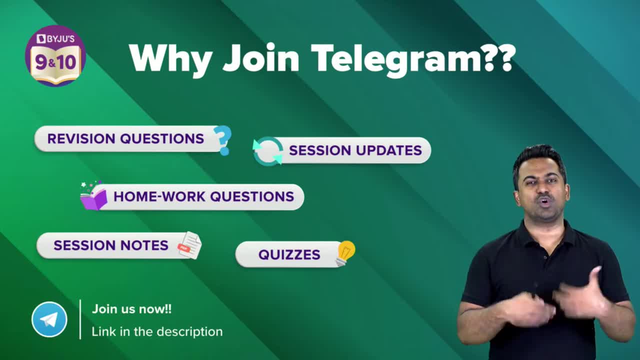 the link to this would be in the descriptions box, because if you're not joining the channel you're missing out on updates related to the session notes. you know the PDF files with the instructors handwriting would be there, which are going to come pretty handy for you when you're. 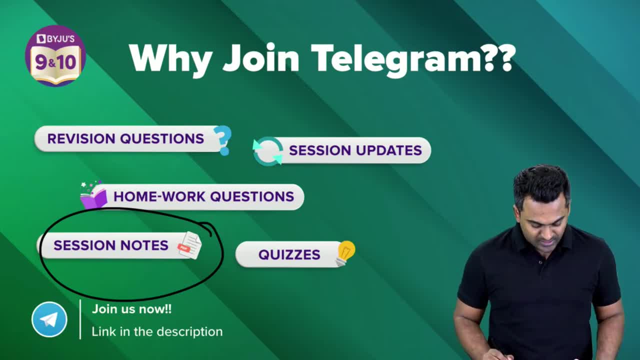 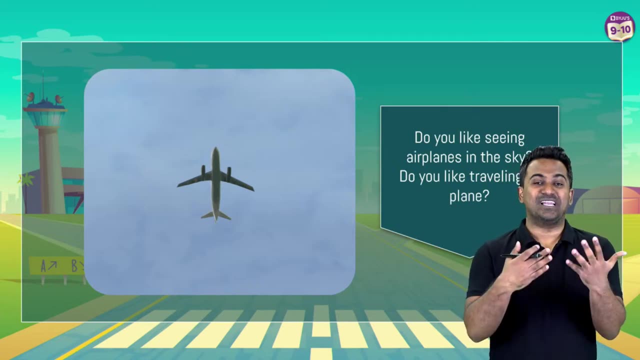 revising all of this stuff later on. all right, so make sure you join the Telegram channel and then quizzes, homework questions, session updates and all the revision questions. yes, so come on, let's start with this session today. I'm sure you like seeing airplanes in the sky. yeah, I'm sure a lot. 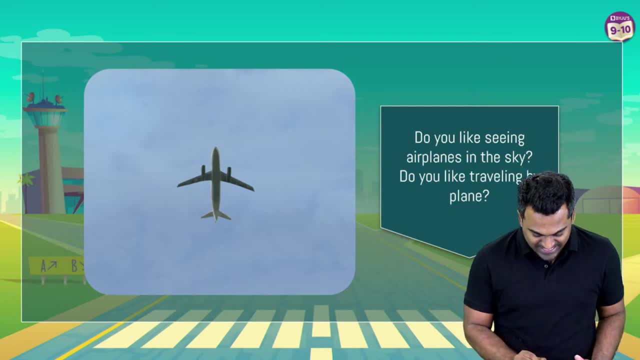 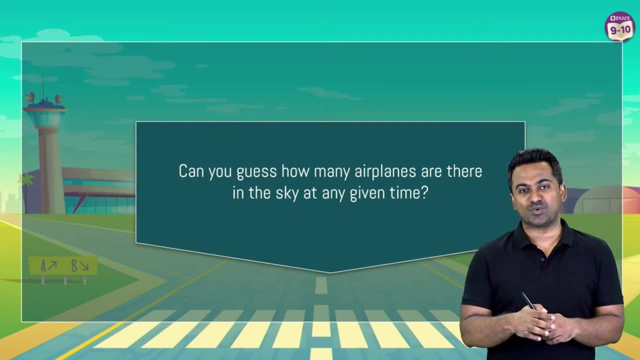 of you must have also traveled with these airplanes. now my question to you is this: can you guess how many airplanes are there in the sky at any given time? because this question must have popped up in your head, like if I'm flying at certain altitude in the sky, are other planes also? 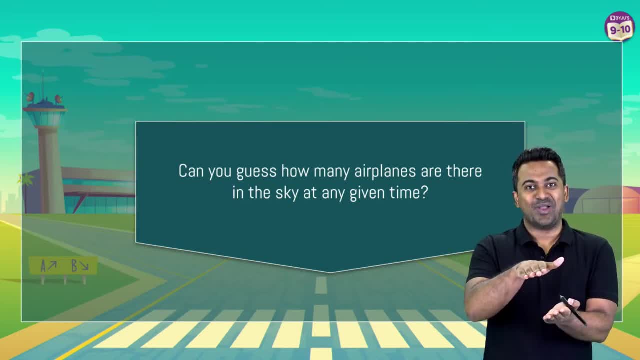 flying at the same altitude, or they're likely above than me or below my plane. what is it going to be? yes, Tatleen says she's not able to join. Tatleen, click the refresh page. I think you know there's some problem with the internet. 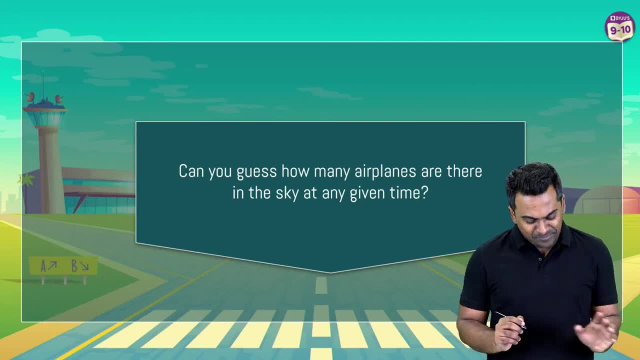 connection you should be able to join. yeah, so how many airplanes would there be in the sky at any given time? Prashant sir says so many. all right, so you've escaped with the accuracy number. Madiha says no idea. it's a hard question, okay. Jyoti says so many- again, a lot, all right, no idea. 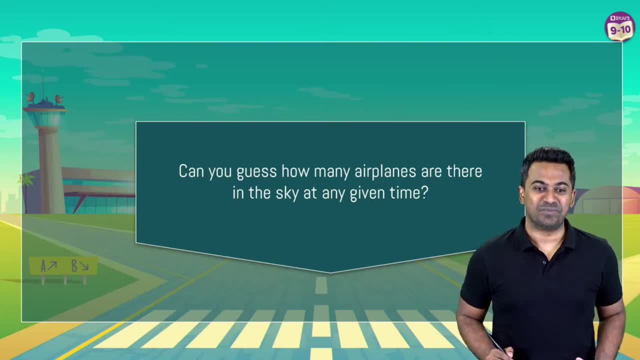 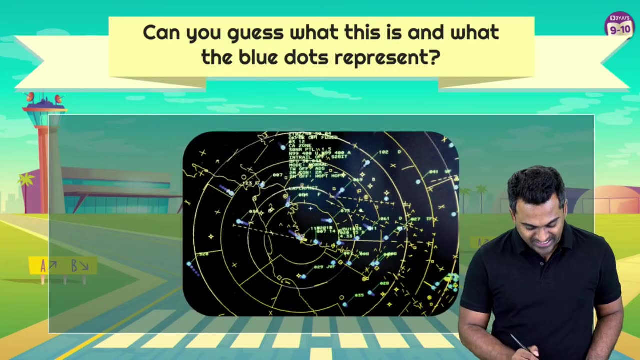 Shivansh says there are going to be many airplanes. Pinky says three. no, Pinky, I think: oh no, it can't be infinity. it can't be infinity. cool, so I'm going to reveal it to you in a bit, but can you? 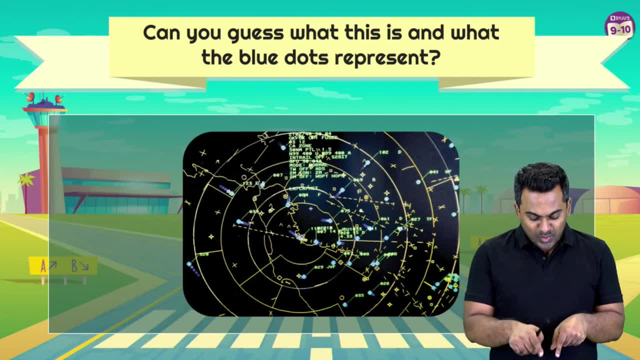 guess what this means. you know this picture. what do the blue dots on this picture may represent? all plane flew at different altitude. it's what Shivansh says: yes, all right. so 10,000 is what your answer. I believe you're closer. is that 10,000, I'm counting. 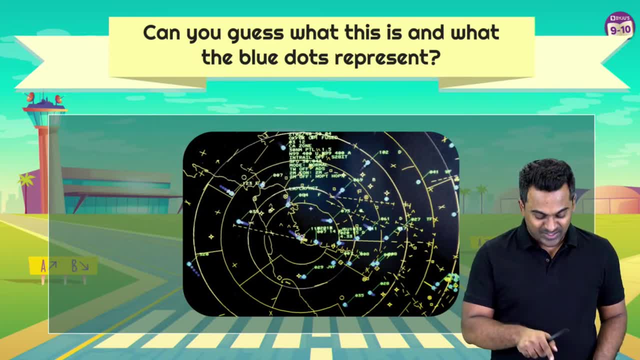 zeroes appropriately, or is that 1,000,000, I don't know all right. so what do these blue dots represent? Pinky Prashant, sir have given the answer: they represent airplanes. yes, so if you. 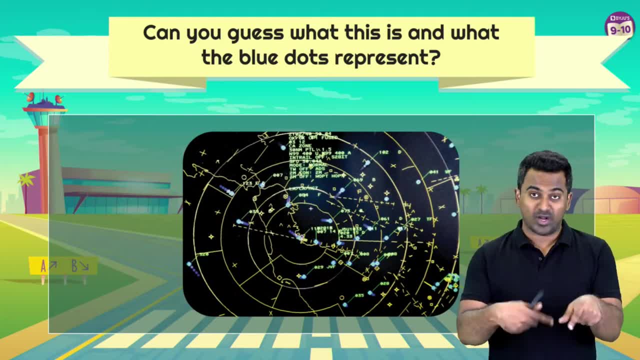 you know, observe what happens at the air traffic control, which I'm going to come in a bit. all these blue dots here represent the plane, right, but they should be representing something else, right. I mean, this should represent what? because this is going to be the heart and soul of 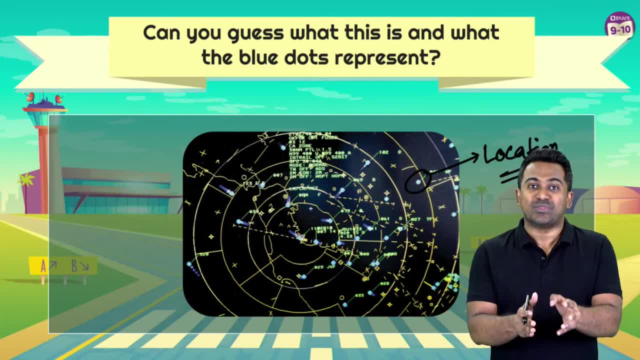 location. but then location is always with respect to some point. yes, because if I say where is your school located, you may come up with an address, but then it is only going to make sense if I measure it with some point like your home. maybe the school is located far away from your. 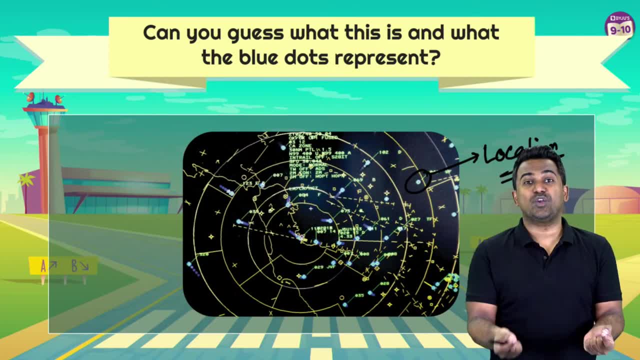 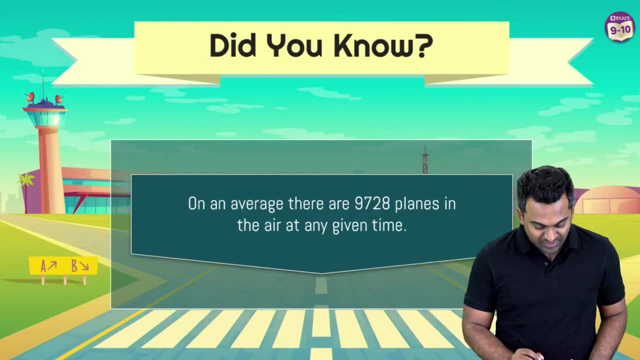 home, or maybe it is located very near to your home, so point of reference is very important. by the way, I'm going to tell you now how many airplanes are there in the sky at any given time average- okay, this is a rough number. they are approximately 9728 planes in the sky at any given. 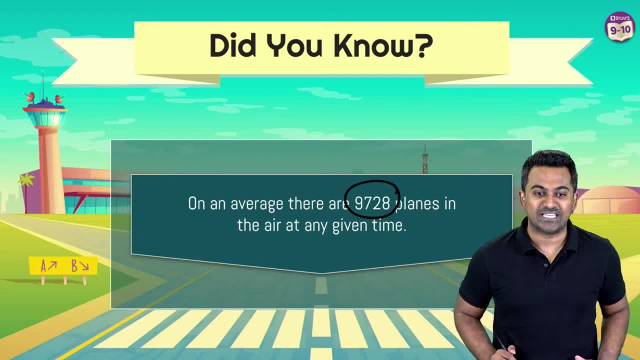 time. okay, Pinky is actually Simran, all right, so I'm going to call you Simran for now. I hope I just remember this. so, as I said, on average they are going to be 9728 planes in air at any given. 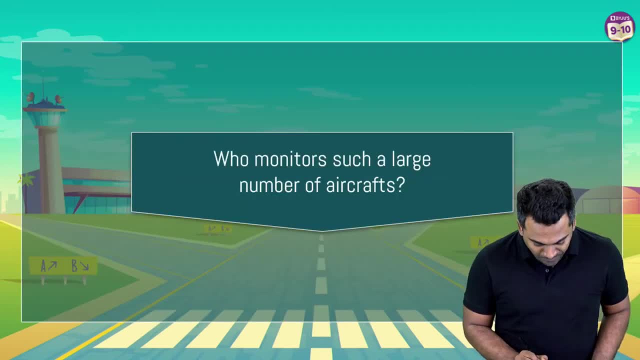 time. so many planes flying- yes, cool. so who do you think monitors such a large number of aircraft? yeah, because there should be some kind of monitoring happening right, otherwise they are going to be crashes. yeah, because some planes may fly at the same altitude. you know, anything can. 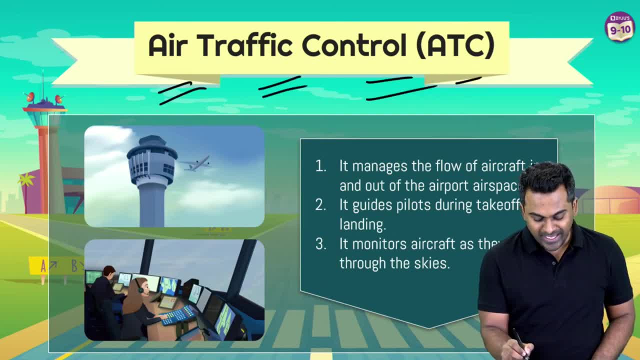 happen. so it is actually the air traffic control ATC which manages the airplane traffic, so the flow of aircraft in and out. so they give instructions, it guides the pilot during the takeoff and landing and it monitors as they travel through the sky. so it's actually the air. 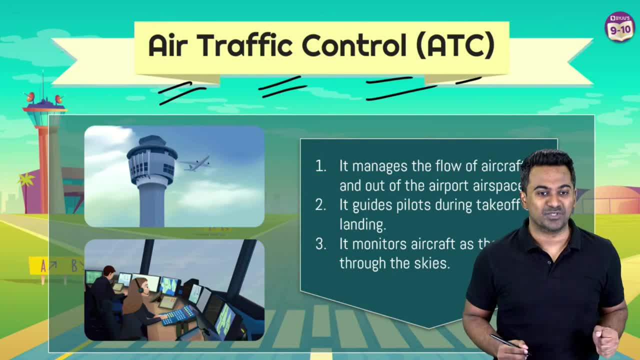 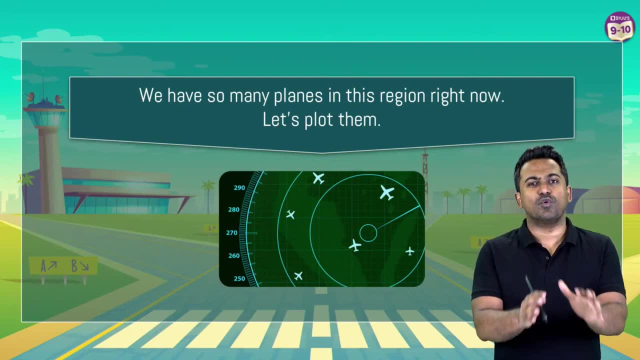 traffic control which does all of that. the air management, like Muskaan, has said out there, all right, so so many planes in the region right now. so the idea, as I said, today's topic is focused on one thing, the heart and soul being location. 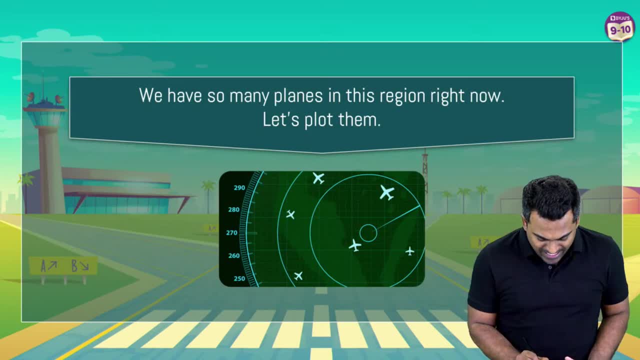 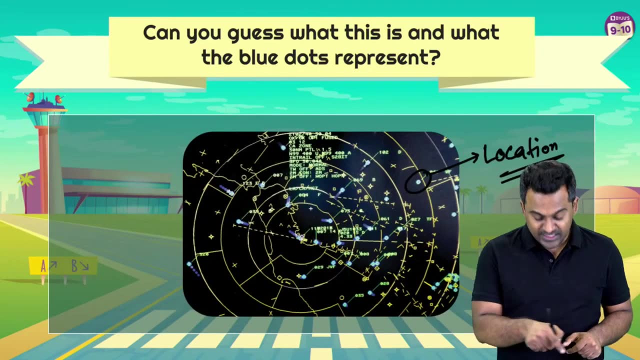 okay location with respect to something. so I'm going to introduce an idea now. okay, as you must have seen in the picture earlier- you know this picture- if you zoom in a little close here you will see this. look, if you zoom in a little closer. 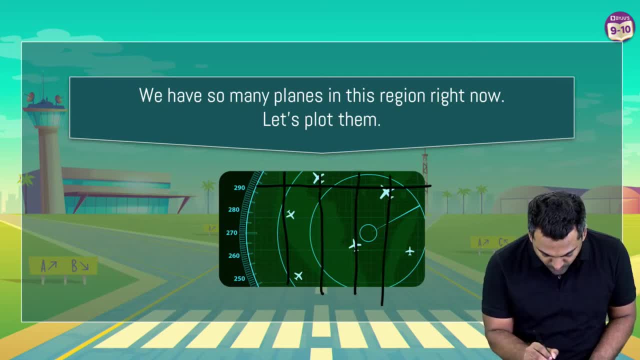 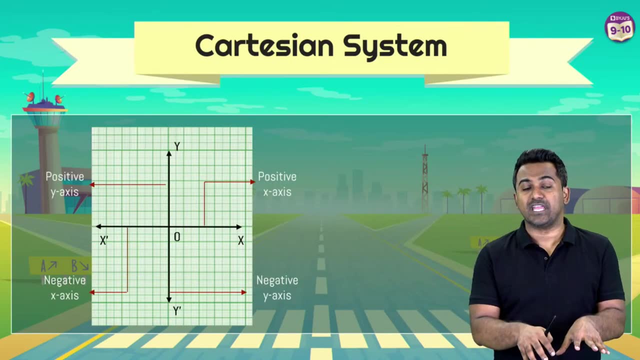 you will see these lines. let me just draw them out in a proper way for you. yeah, so this is how we locate these planes on a coordinate plane. so that's the reason why we are studying this, called as the Cartesian system, probably one of the best inventions in the history of math, because it is 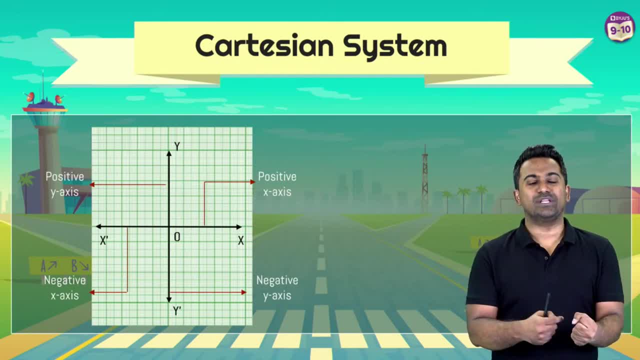 this Cartesian system or the coordinate plane, which gave us a reference, of converting problems of geometry into algebra. Okay, so this forms the bridge connecting algebra and geometry. all right, so let me just acquaint you with what this is. so, as you can see, you have this. let me just change the color a bit. 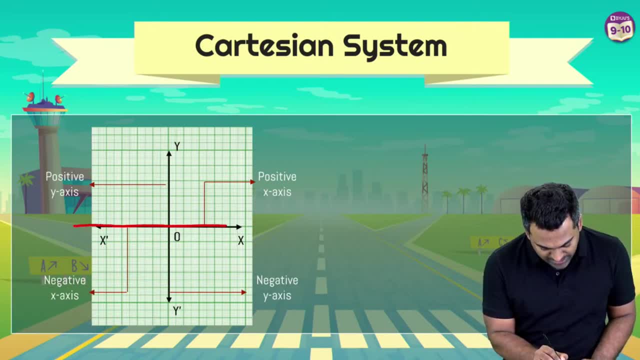 okay, what do I take? right? yeah, so this line that you see, the horizontal line, is called the x-axis and this vertical line that you see here is called the y-axis. all right, and this point where the x and the y-axis are intersecting or cutting one another. 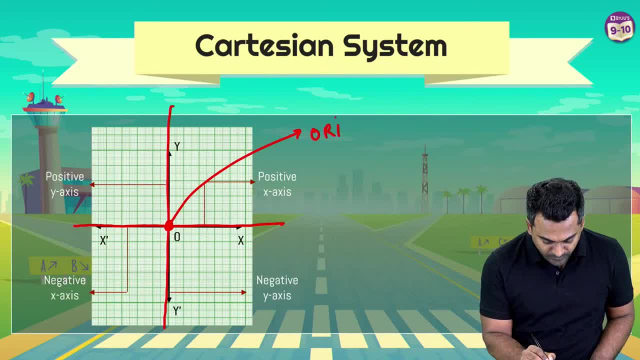 this point is called the origin. all right, so the horizontal line is called the x-axis, the vertical line is called the y-axis. the point where the x and the y-axis are cutting each other is called the origin. all right, now to the right side of now. I want you to imagine this as a 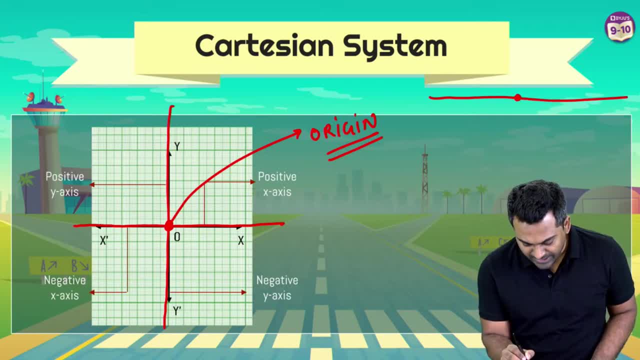 number line. all right, number line. I'm sure you guys are familiar with the number line. right you have zero, and to the right-hand side you have one, two, three, four, five and to the left-hand side of zero, what do you have? you have minus one minus two, minus three minus four. yes, 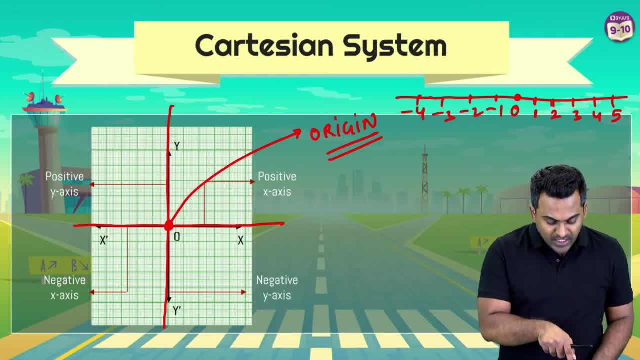 you guys have studied the number line, right. so imagine this origin to be zero. all right, then the right-hand side of zero, you will have all these positive numbers- one, two, three, four, five- and to the left-hand side of zero, you will have the negative numbers, right? so that's the. 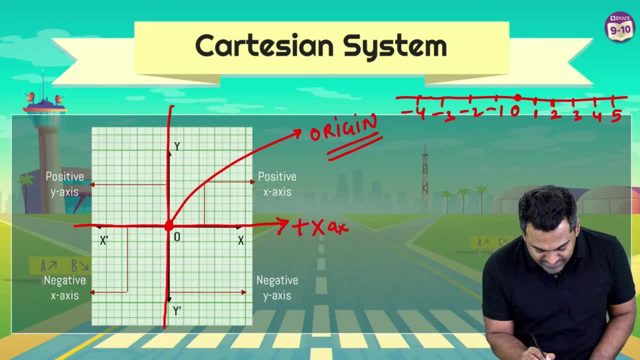 reason why this is called as the positive x-axis to the right side of origin, and the one to the left side of origin is called as the positive x-axis, So negative x-axis. okay, this should be pretty clear now. yes, look, x is horizontal, y is. 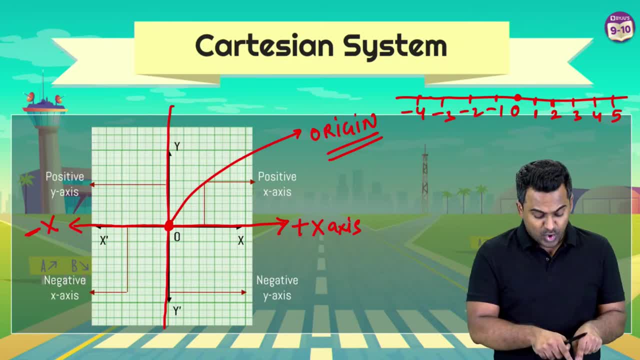 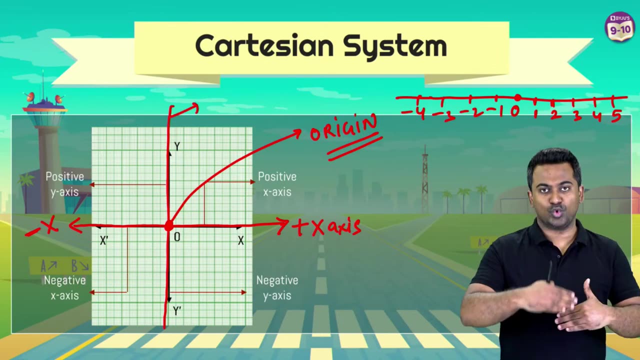 vertical. the point where x and y are cutting is called the origin right. and now to the right side of origin, you have your positive x-axis. to the left side of origin, you have your negative x-axis, similar to the number line. okay, and then top bottom. so this to the top of origin. 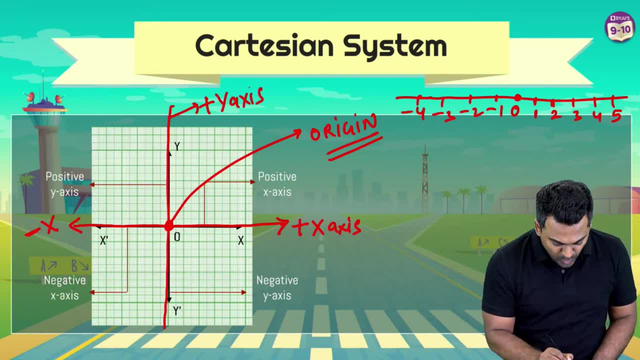 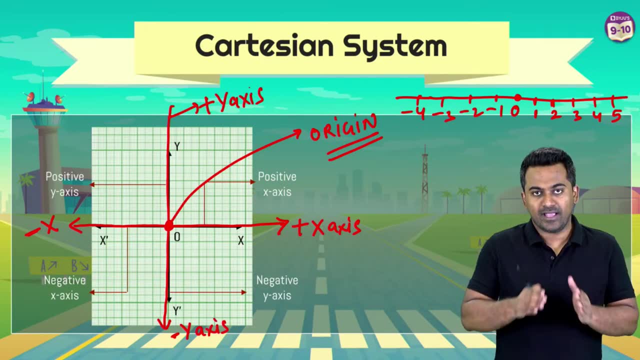 this is going to be the positive y-axis and below the origin you will have your negative y-axis. okay, I hope this is crystal clear. yes, right plus left, minus up plus down, minus. okay, because this is going to be very crucial. 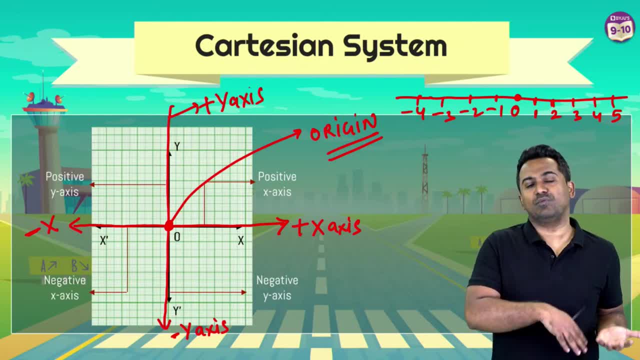 guys, you need to be able to understand this. only then you will be able to understand how will you plot points on a coordinate plane, particularly. you know how do you check the location of a point. okay, so I hope this is very useful. 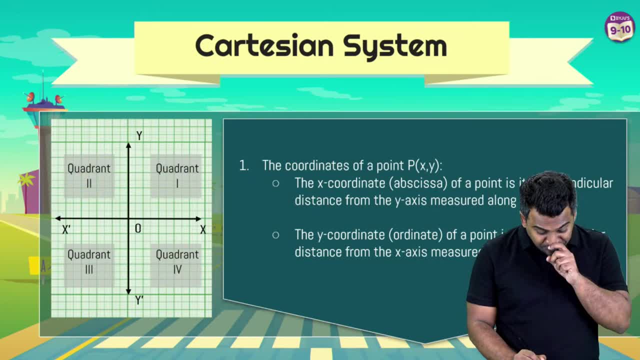 Very clear. yes, very basic. come on next point. there are certain technical terms that you should get acquainted with. you know the x-coordinate. there is another name for this, we call it abscissa. okay, the x-coordinate is called the abscissa and the y-coordinate is called the. 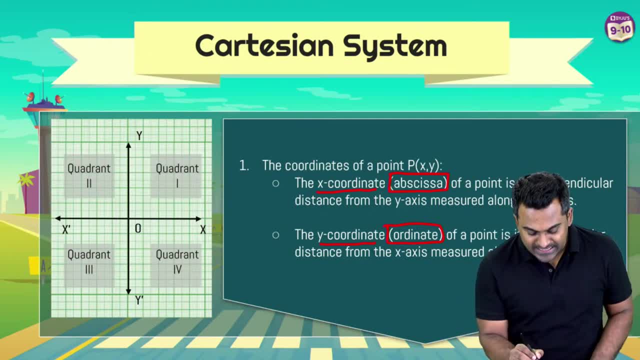 ordinate and any point is written in the form of x- y. first you have x, then you have y, similar to the way you read it alphabetically as well. Alphabetical order: first comes x, then comes y. okay, now this region here is called the first. 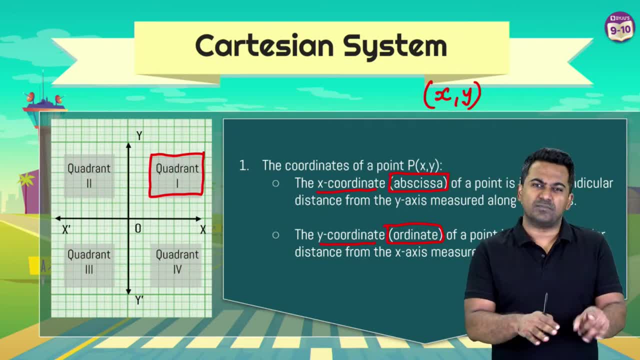 quadrant. I'm just making you aware of the technical terms and then we're going to jump to the fun part. okay, so in this first quadrant, as you can see, this is what this is positive x. yeah, the line that I've just drawn, and this is what positive y: yeah, this is positive x. 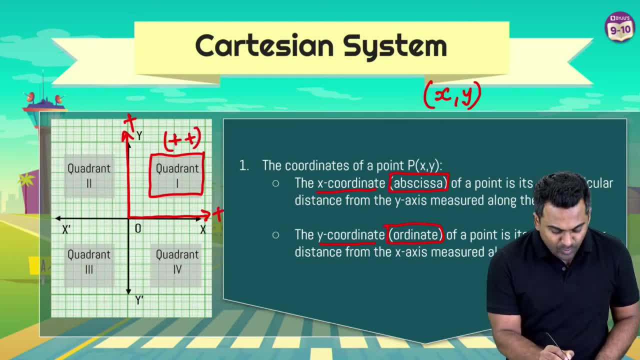 and this is positive y. so in first quadrant both x and y are, say I say, are positive. okay, now this is the second quadrant. right in the second quadrant, what is x-axis? here, You've just learned it. we call this negative x-axis. so this is what: negative x, positive y. 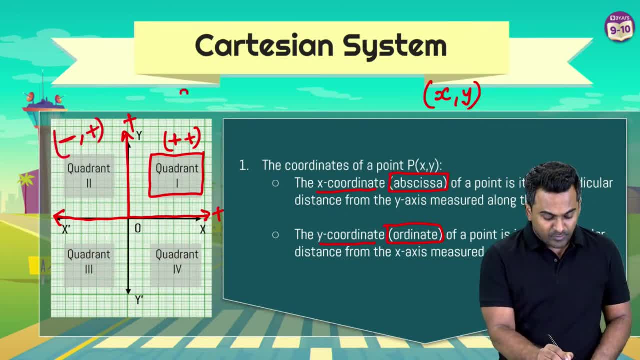 so minus plus. I'm writing it in the form of x- y. okay, in the first quadrant x is positive, y is positive. as you can see here, this is the positive x-axis and this is the positive y-axis. 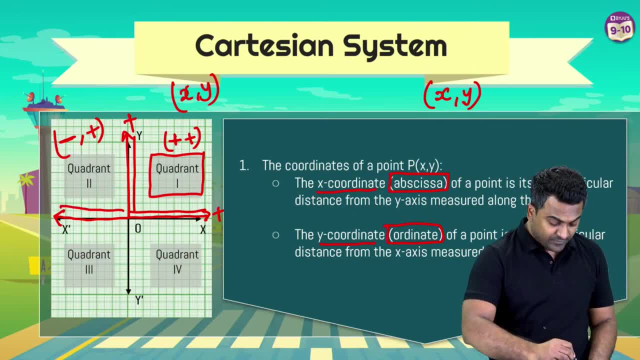 yes, in the second quadrant you have this x-axis, which is negative, and this y-axis, which is positive. if I take a different color now, all right now in the third quadrant, you will see this is the negative x-axis. 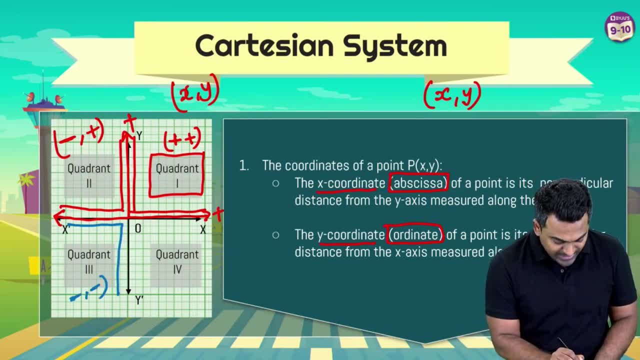 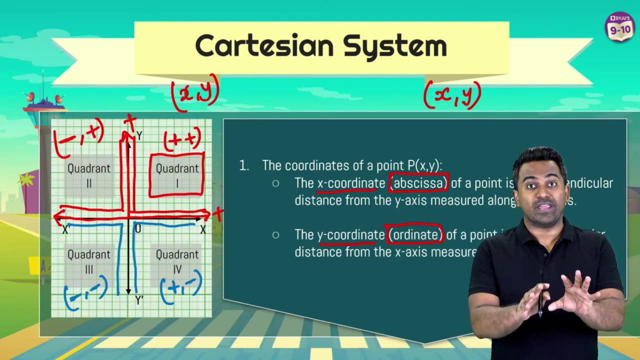 and this is the negative y-axis. yeah, so this is going to be minus, minus, and in the fourth quadrant, if you observe, you have the positive x-axis and the negative y-axis. so points here are in the form of plus, minus. so these are basics. I hope we have understood them. 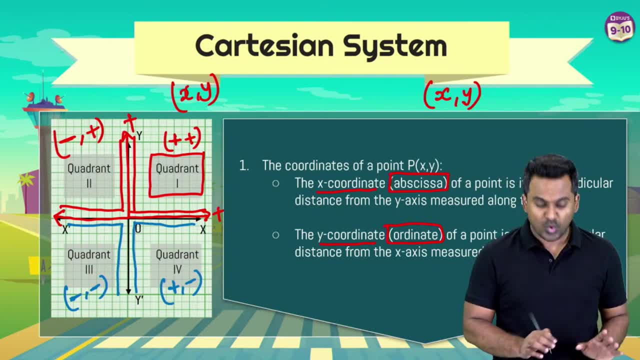 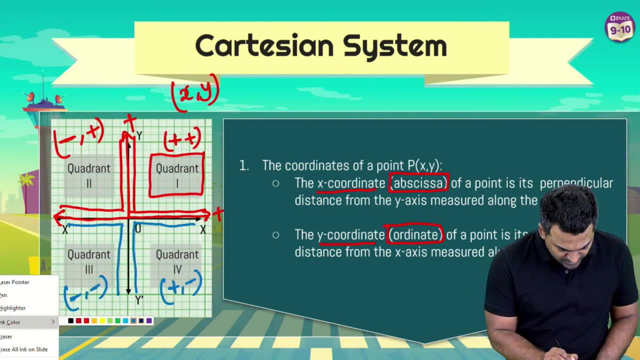 right, come on. let's move on now and check it out. so I hope this is crystal clear. first quadrant: both x and y. let me just write it down here for you with a slightly better color for you. okay, so in the first quadrant it is x positive, y positive. 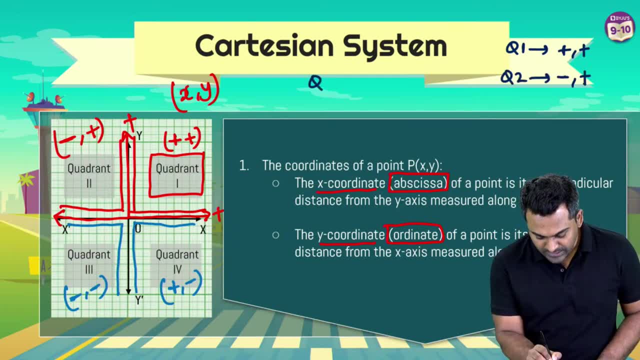 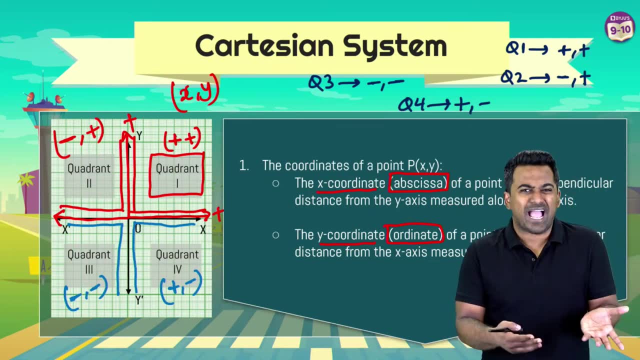 in the second quadrant, x negative, y positive. in the third quadrant, x negative, y negative, and in the fourth quadrant, x positive, y negative. you shouldn't actually have to memorize this. it is quite logical the moment you check out the direction it is happening in the anti-clockwise. 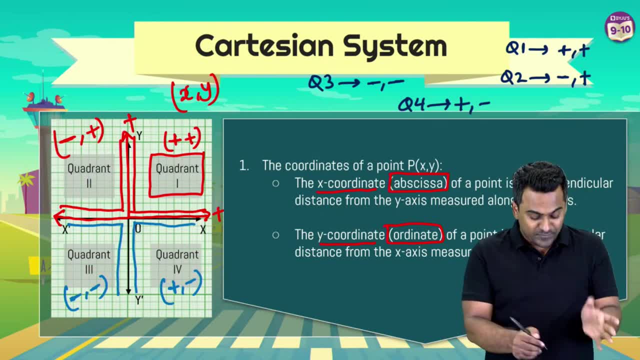 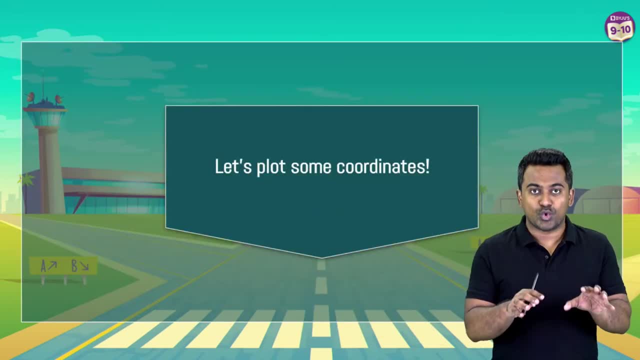 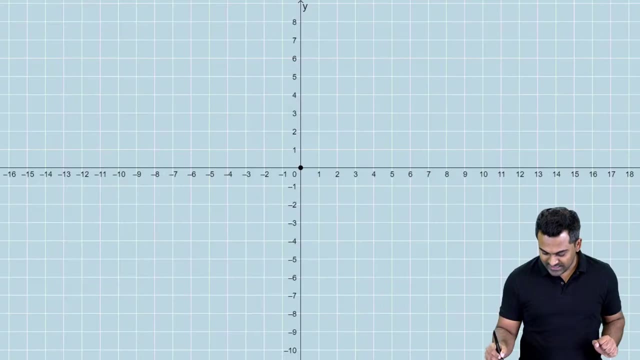 because what we are going to learn in this session today is how to plot points on a coordinate plane. that's it all right. come on, let's jump over and check out how this is to be done. all right, so I hope this is visible. yeah, as you can see this dot in the middle. 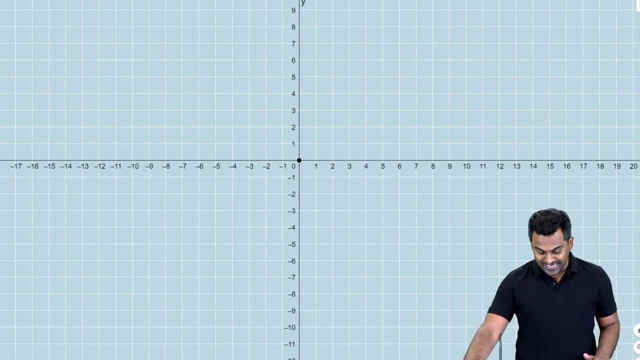 yeah, this is going to represent the origin: the right-hand side positive x, the left-hand side negative x. up you have positive y, down you have negative y. come on, let's take the example of a point. let's say I want to plot 1,, 6, x1,, y6,. I repeat it again: I am trying to plot. 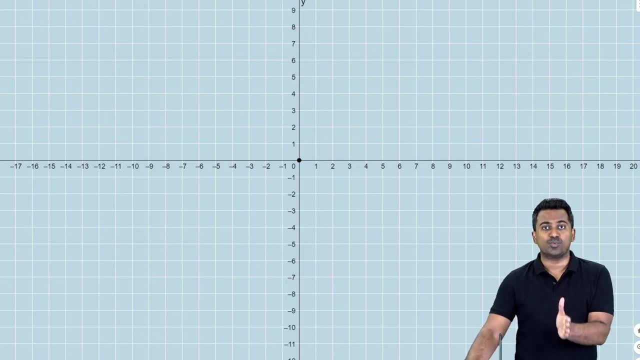 the point 1, 6, which means x is 1, y is 6, where will that be? look, x1, y6, so you see, this is where the point 1, 6 is going to be. yeah, you move 1 on the right. 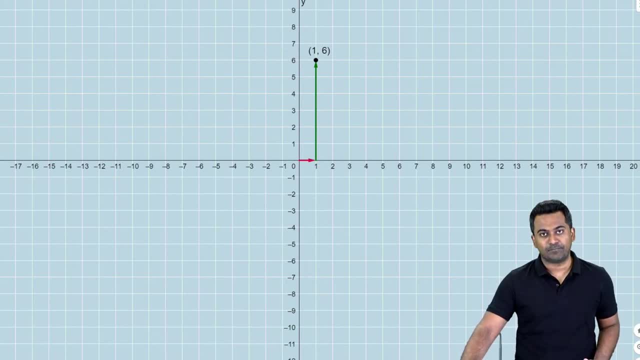 because x is positive. and then you go up by 6, and you reach the point 1, 6,. yes, so you've understood how do we plot point 1, 6,. you always start from the origin, look. 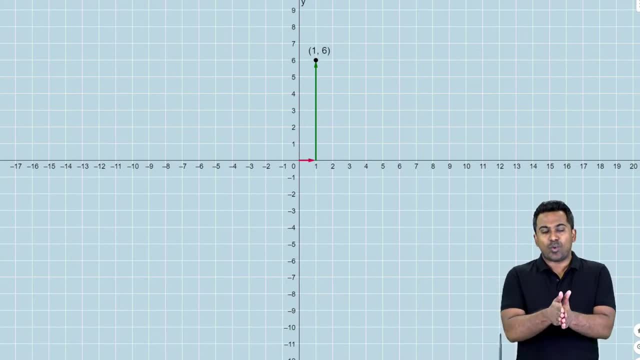 you always start from the origin. and then x is 1, so you move right by 1, y is 6, so from here you go up by 1,, 6, so you reach the point 1, 6,. you always start from the origin. 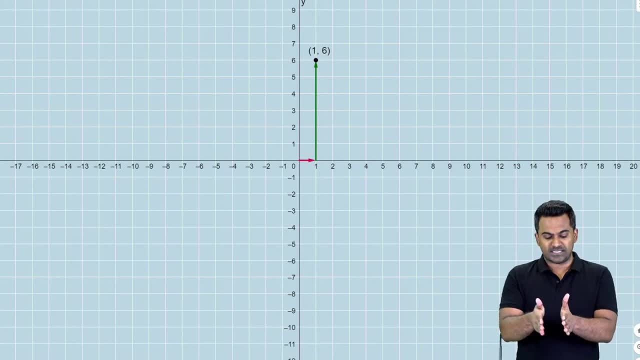 you go up by 6, okay, so this is going to be 1,, 6,. from the origin, x is 1, you move right by 1, and from here you go up by 6,. come on, let's change the point now. let's suppose 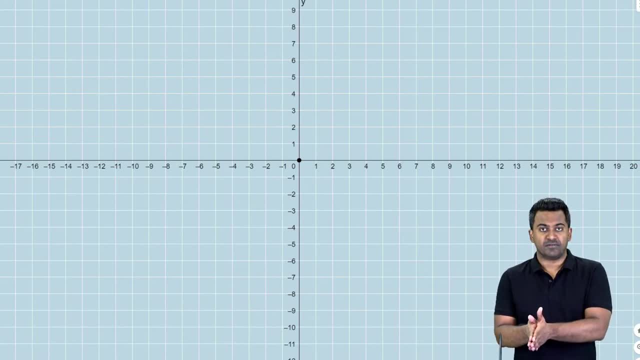 now I'm trying to plot 6, minus 5,. x is 6, y is minus 5,. I repeat it: x is 6, y is minus 5, let's plot it so from the origin. I go right: x is 6, so I move right by 6,. 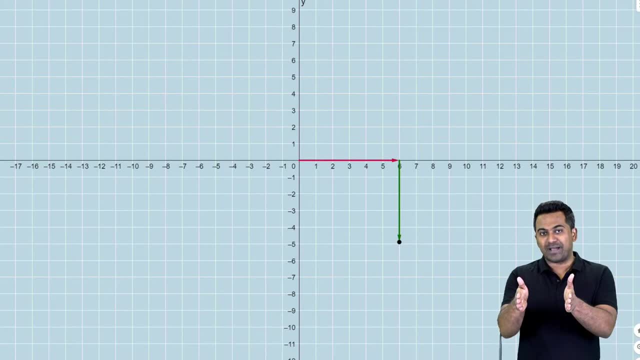 and then, how much is y minus 5,? so y is minus up or down. y is minus down, right, so I go down by 5, and this is going to be what: 6 comma minus 5, is that clear? so you just need to remember. 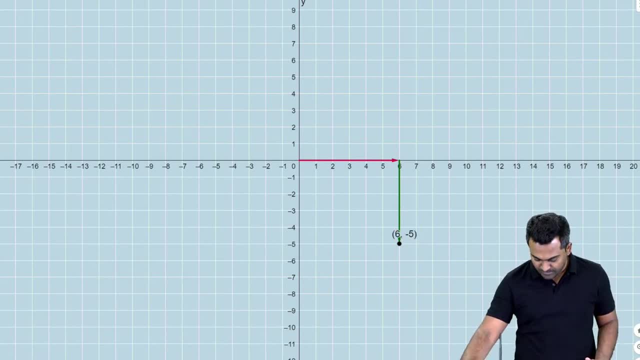 we're always starting from the origin. that's it. let's take a new example. let's suppose this time I want 8 comma 4, x is 8, y is 4, so from the origin I go right by 8,. right because x is. 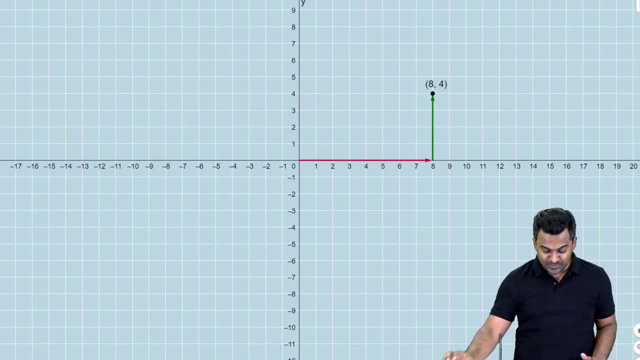 positive, and then I go right by 8, because x is positive, and then I go right by 8, because x is 4, because y is positive as well. so this will be 8 comma 4,. new example, let's suppose this time. 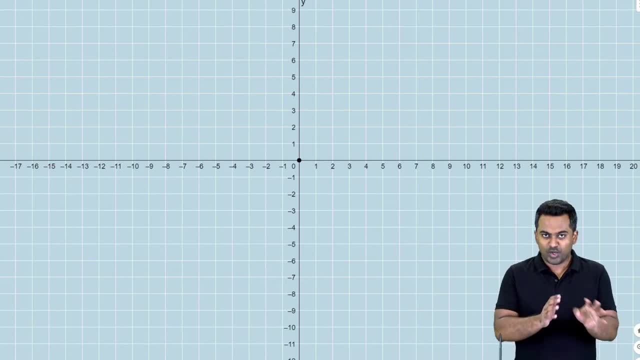 I want minus 6 comma, minus 8, okay, are you able to hear this? minus 6 comma, minus 8, x is minus where I'll go right or I'll go left. I'll go left, yes, because on the left it is negative. 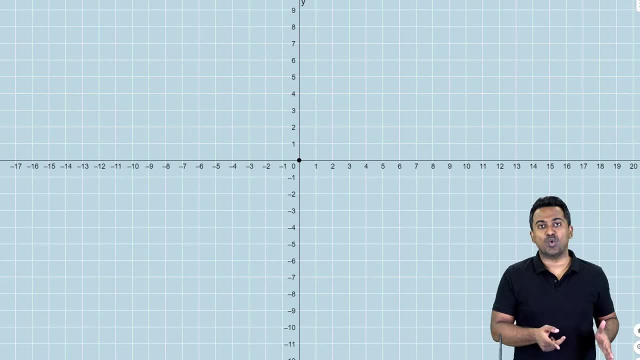 minus 6,, minus 8, so y is also minus, which means I'll go down. this is all you need to remember. right hand side x positive, left hand side x negative. up y positive, down y negative. that's it, okay, let's plot the point now. minus 6, comma, minus 8,. 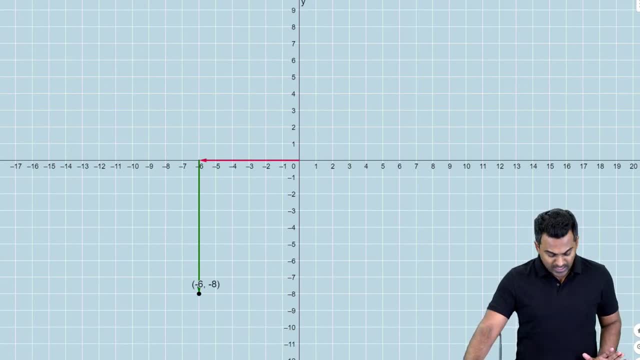 so minus 6,, minus 8,. okay, so I've gone left here by minus 6, and I came down by minus 8, so this is where minus 6 comma minus 8 will be. and now let's suppose I want to plot. 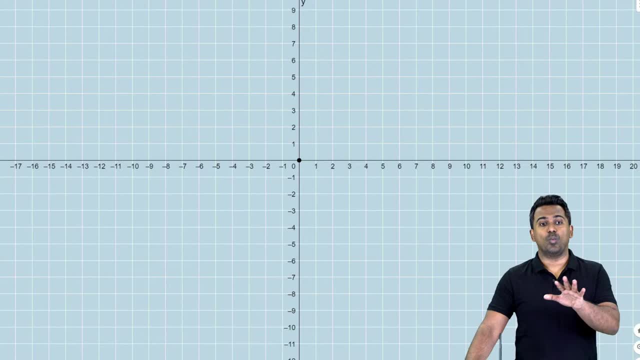 10 comma minus 2, x is 10, y is minus 2, so let's check this out: x 10, y minus 2, so x 10, y minus 2, 10 comma 2 means I'll go up by 2, but since this is 10 comma minus 2, I've gone down by. 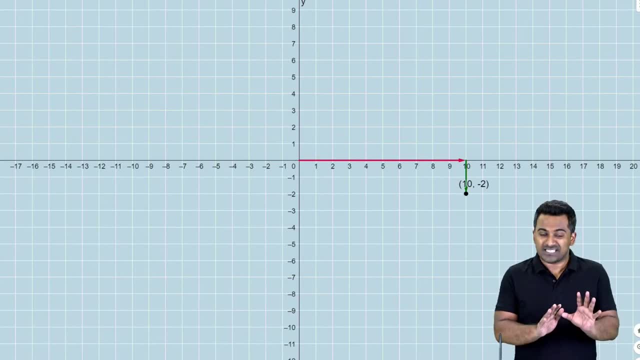 minus 2, so I hope this is interesting. yeah, I hope this is understood. understood, that's, that's more important. yeah, one, one last example, and then we will go and proceed to this. all right, so this time we want to plot 5 comma minus 8, let's say, okay, so x 5, y minus 8,. 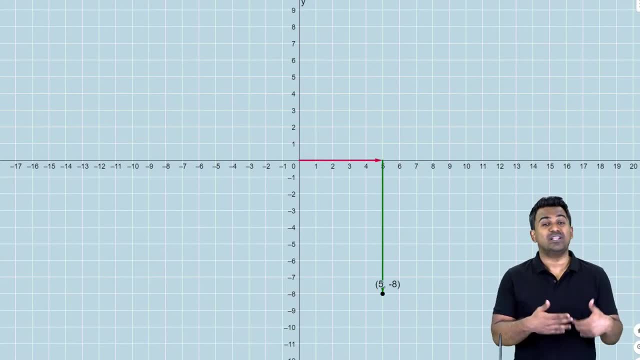 so all these points that you've been plotting could be considered to be the location of the planes right on on. maybe ATC also has a screen like this and all these points that you see here can represent the location of a plane. right, and we can do wonderful things right, we can find out. 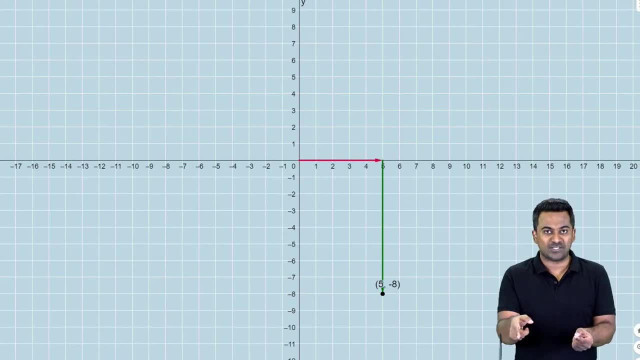 the distance between two planes. I'll show you how to get the distance formula as well. we can find the midpoint of of those two planes. we can find the equation as well. if we want to. plenty of exciting stuff could be done, as long as you've understood these basic fundamentals. 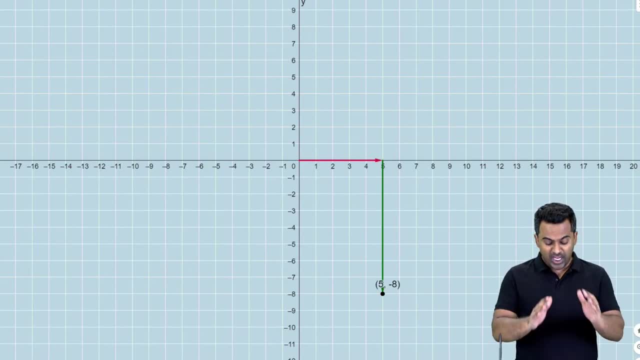 okay, everything starts with the basic. guys always remember this: if you're good with the basics, you can pretty much master any topic. one last example. and then we're going to go on: 10 comma 5, x, 10, y is 5, yeah, minus 4, comma minus 5, x minus 4, y minus 5,. 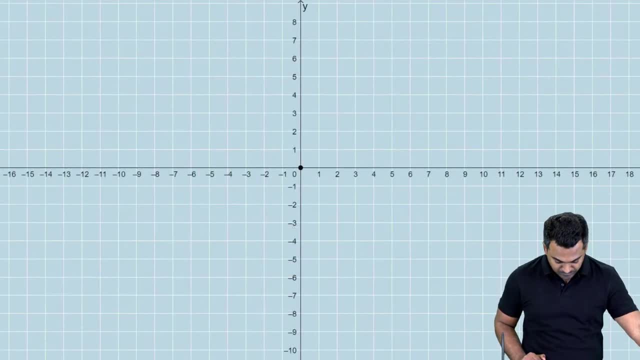 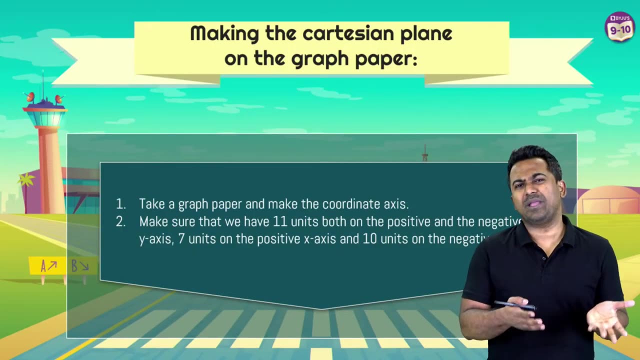 I hope this is understood. come on, let's move on and check out our topic. all right, cool. so it's time for us to plot coordinates now. for you to be able to do this, you need a graph paper. yeah, if it is not there today, with you, it's absolutely fine. 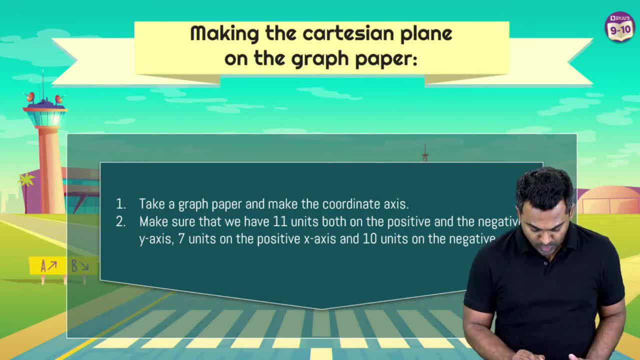 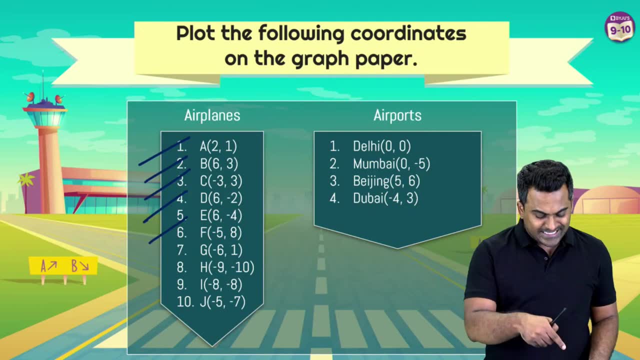 you can understand this and then plot it on a graph paper later on. right, as I said, these can represent these points that you see here. okay, all of these coordinates can be represented by airplanes. and all of these coordinates, like Delhi, is represented by 0 comma. 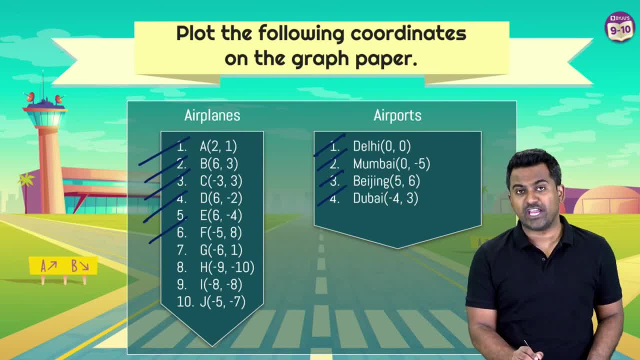 0, Mumbai is represented by 0 comma minus 5, Beijing, 5 comma 6, Dubai minus 4 comma 3, these can be represented as airports. all right, come on, let's move on now and plot these points. 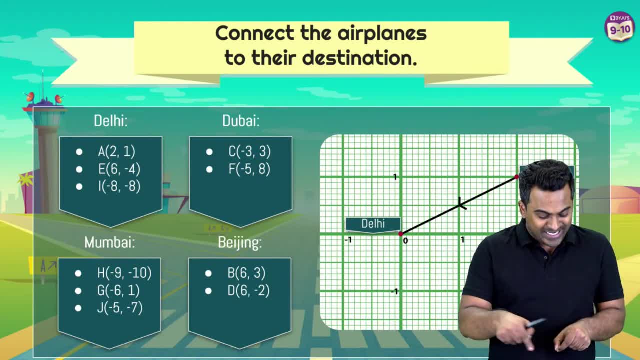 okay. so we've got to. what do we do? connect these airplanes to their destinations like, let's suppose, Delhi airport- these are the destinations. Dubai airport- these are the destinations. so, as I said, plenty of exciting stuff could be done. come on, let's plot it now. 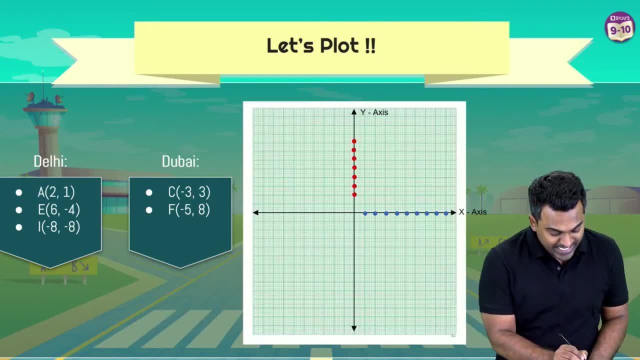 all right. so I want to plot a first. what is a here? 2 comma minus 1, so this is going to be what this is going to be. 0, is 1, 2, 3, 4, 5, 6,, 7,, 8, 9.. So this is what Positive x And this is going to be what. 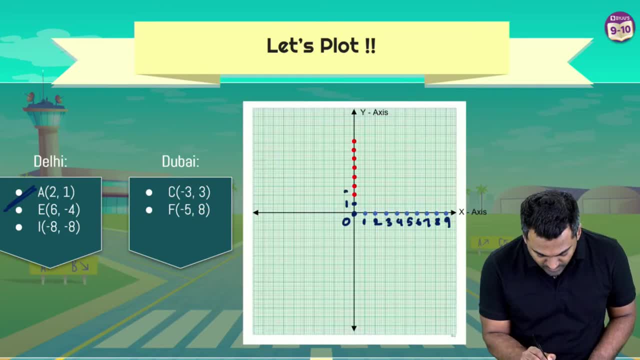 1.. Okay, let me just write it on the left hand side: 1, 2, 3, like that. Okay, so I'm going to rub this. all Okay so now, where 2, 1 will be x2, y1.. So this is where a will. 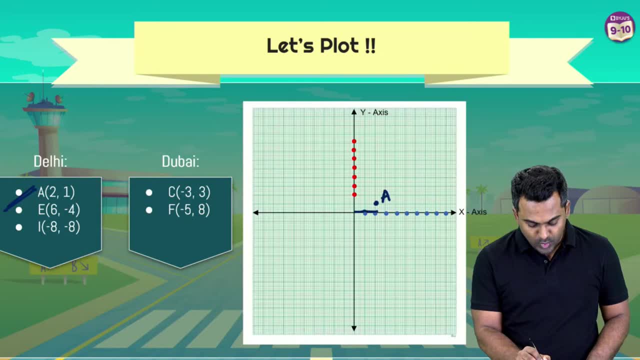 be right: x2,. so look 1,, 2, and y1.. All right, so 2, 1 will be here. So this is a. I'm writing that out Now: 6, minus 4.. I'm trying to plot e: 6, minus 4.. So where is? 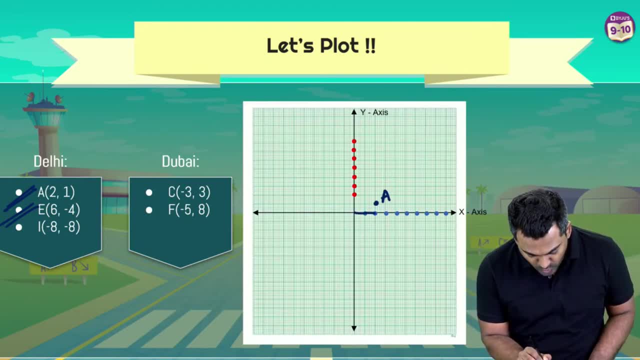 x6?? I go right by 6.. 1,, 2,, 3,, 4,, 5,, 6, right. And now minus 4 means what do you do? I come down, right, Come down by 4.. 1,, 2,, 3,, 4.. So this is going to be. 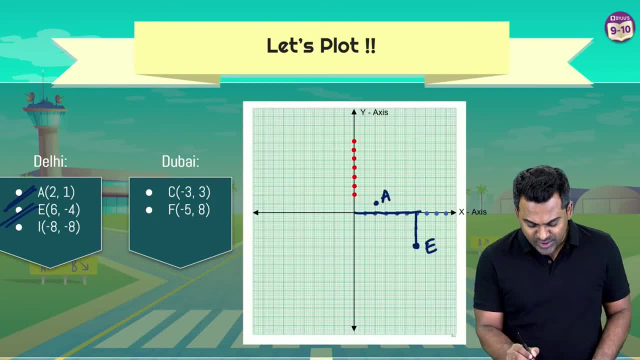 e, 6, minus 4.. You just need to remember the directions. This direction is positive, This direction is negative, This direction is positive And this direction is negative. So this is negative: y plus y plus x minus x. That's all, Okay. Yes, this is going to. 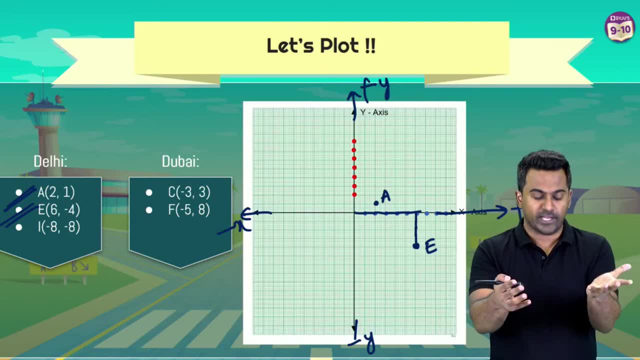 be there in class 10 as well, but in a little bit more detail. Okay, i minus 8,, minus 8.. Now minus 8, I go left by 8.. So 1.. 2,, 3,, 4,, 5,, 6,, 7,, 8.. So this is it. And then minus 8, y as well. So I go down, I don't go. 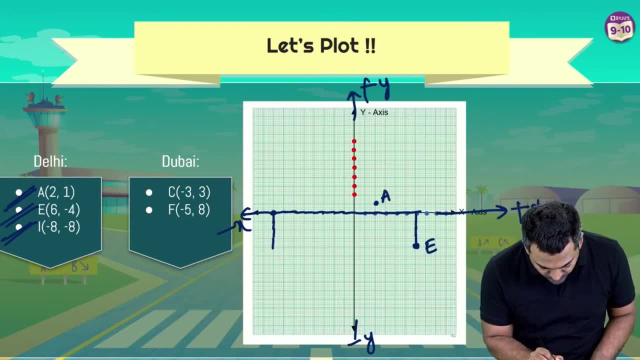 up right. So 1,, 2,, 3,, 4,, 5,, 6,, 7,, 8.. So this is the point i You're understanding this. now, How are we plotting? Because from today's chapter, this is the only takeaway, You guys. 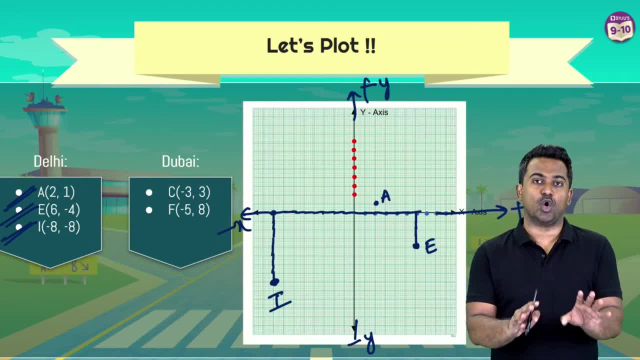 should get perfect with plotting Any point on the coordinate plane. As simple as that. All right Now. c minus 3, minus 3.. Where is minus 3?? I go left And then plus 3, right. So minus 3, minus 3.. This is representing. 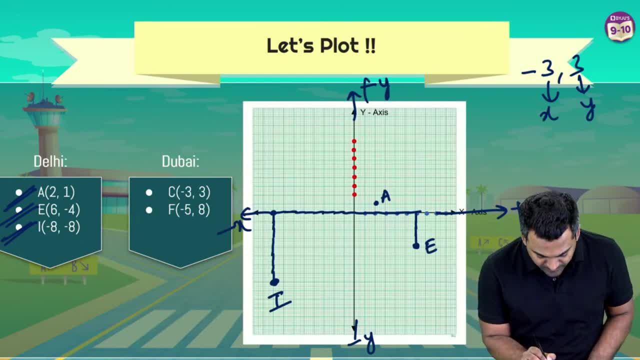 x. This is representing y, x minus 3.. So I go left. So this is going to be 1,, 2, 3.. Yeah, And then y 3 means I go up 1,, 2, 3.. So this is going to be c. Yes, Well done. And now. 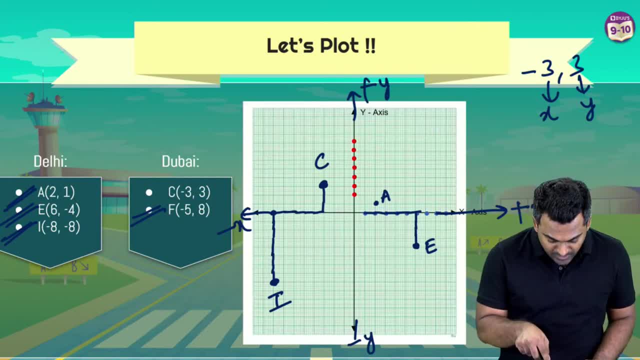 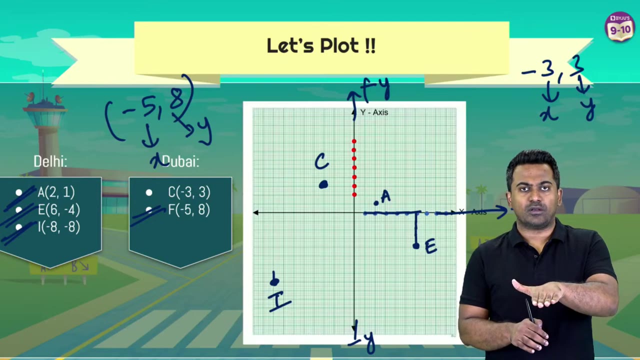 last thing: Minus 5, comma 8.. Yeah, Let me just rub these out: Minus 5, comma 8.. Again, x is minus 5.. Right, Minus 5, comma 8.. So this represents x, This represents y. So x minus 5 means what Left or right? 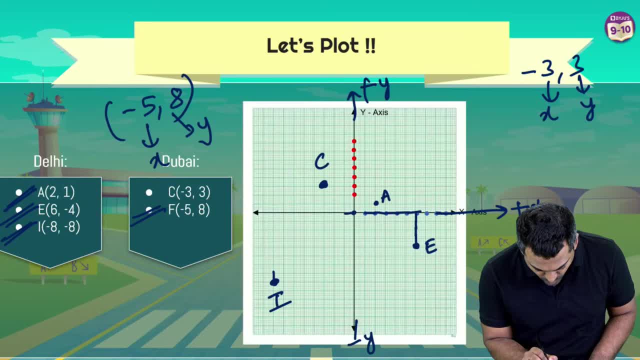 I go left, right, So by 5.. So from this point, origin: 1,, 2,, 3,, 4,, 5.. So this is minus 5.. And now 8 means what? Plus 8, right, So I go up, I don't go down, So from here 8.. 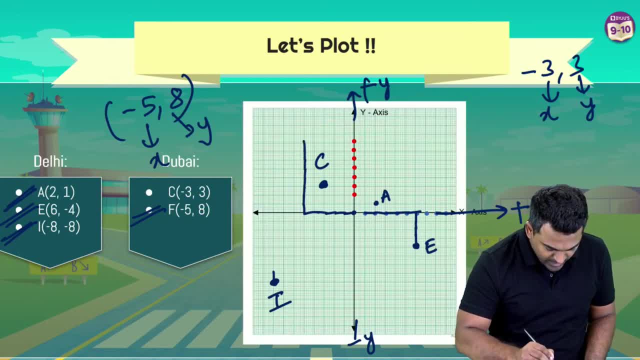 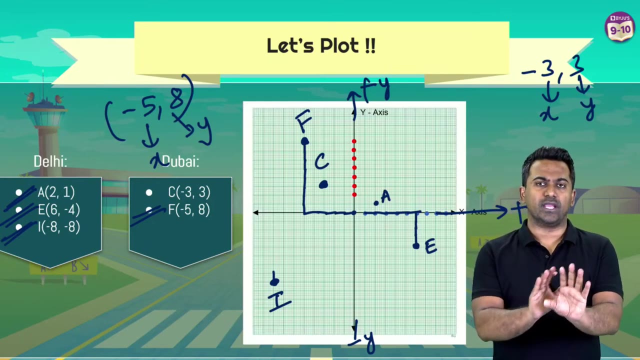 3, 4, 5, 6, 7, 8. so this point will be here. okay, F will be here. that's it, guys. this is how you plot points on a coordinate plane and, as I said, today's topic. you only learning this one very important thing and nothing else. so have you. 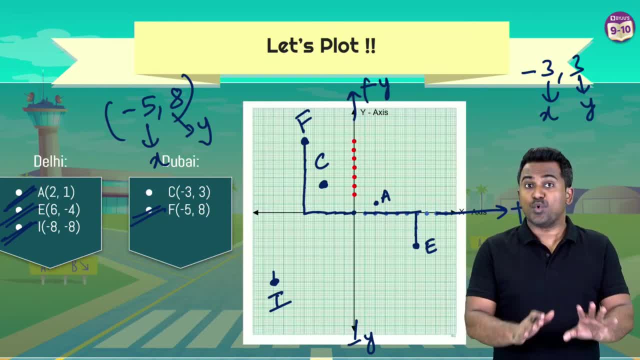 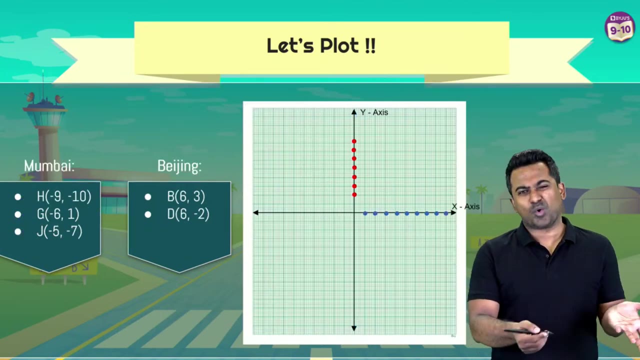 understood this, because this is where everything starts. if you know this, trust me, the rest of the coordinate geometry will flow very, very easy for you. this is the basic that you've got to know: how to plot points on a coordinate plane. I'm sure you've understood this right, so come on, I'm not gonna plot all the 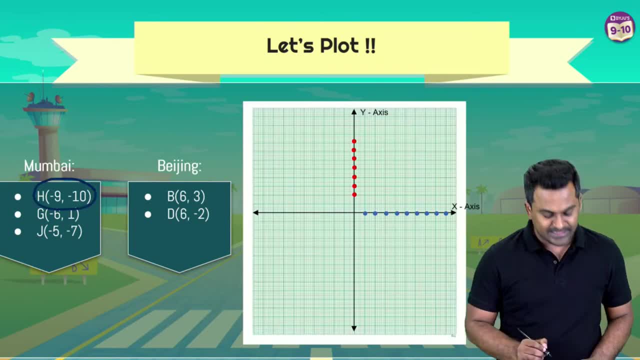 points. now I'm just gonna handpick a few. minus 9, comma, minus 10, let's say: all right, so X minus 9, Y minus 10, so left and then down. so from here I bore 9, 1, 2, 3, 4, 5, 6, 7, 8, 9, so this is 9 minus. 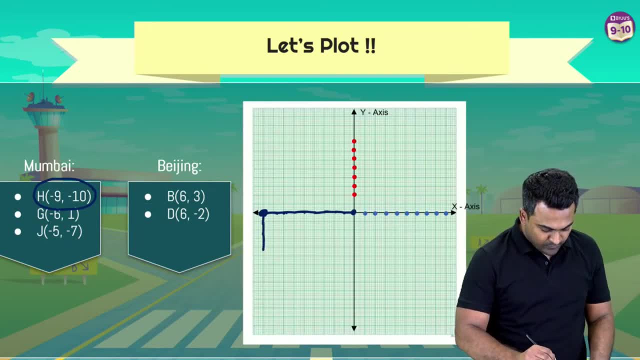 10. so from here I bore 9: 1, 2, 3, 4, 5, 6, 7, 8, 9, so this is 9 minus 9, so this is 9 minus 9 and now minus 10 down. so 1, 2, 3, 4, 5, 6, 7, 8, 9, 10. okay, so this point here is going. 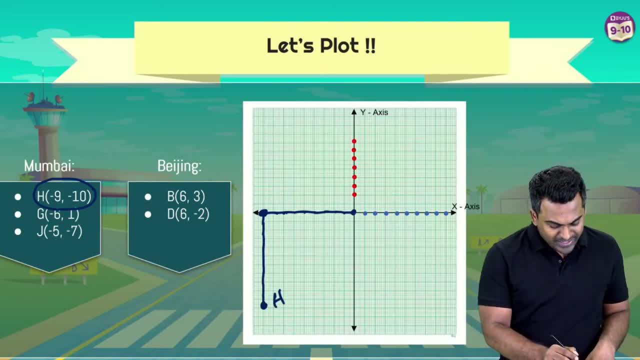 to be minus 9 comma minus 10 and now minus 6 comma minus 1 will be here right. second quadrant: minus 5 comma minus 7 will be here. third quadrant, 6 comma 3. first quadrant, 6 comma minus 2, second quadrant right, sorry. fourth quadrant. 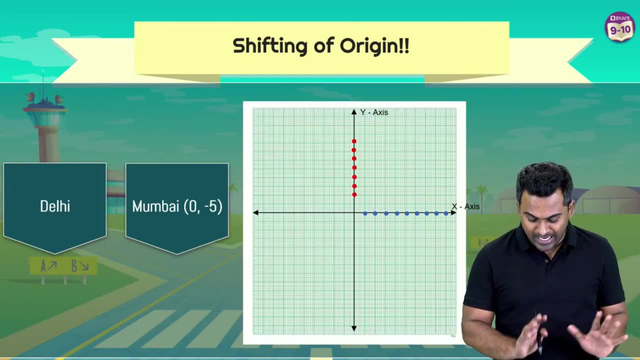 yeah, so this is how we plot points now. now we come to an important thing. the topic was a missing airplane, right? cool. so this is understand this. where is the origin? now, this point is the origin, right? let's suppose this origin is a Delhi Airport. this represents. 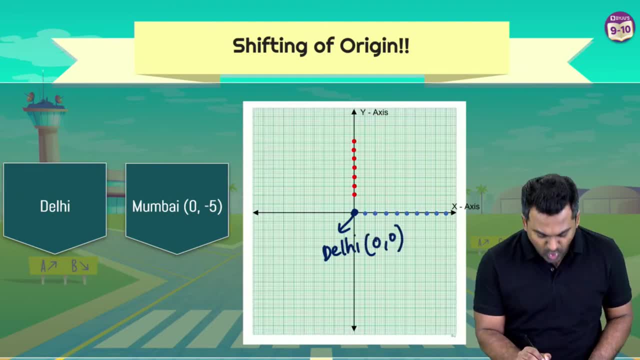 the Delhi Airport and what are the coordinates here? origin means what? X 0, Y 0, because both X and Y are cutting at this point. yes, very good, so this is the Delhi Airport. now let's say Mumbai is where Mumbai is X 0 Y minus 5 X 0. where. 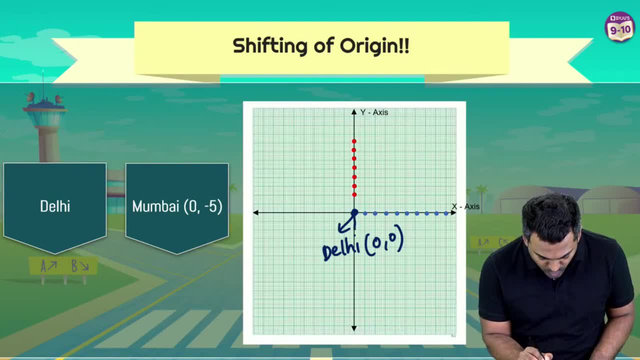 here Y minus 5, I go down. so 1, 2, 3, okay, let's just make it plus 5 to just, you know, not get clumsy. that's all. so one, two, three, four, five. so this will be Mumbai airport, right, which is what? zero comma, five. yeah. 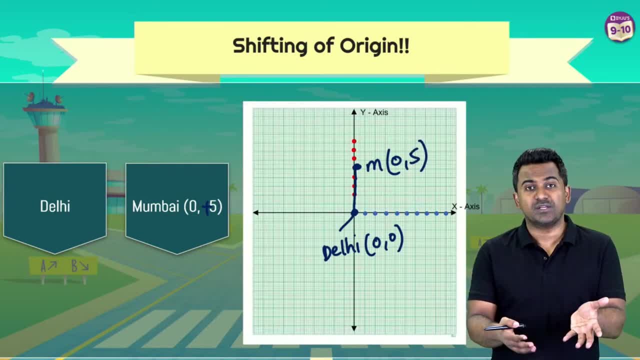 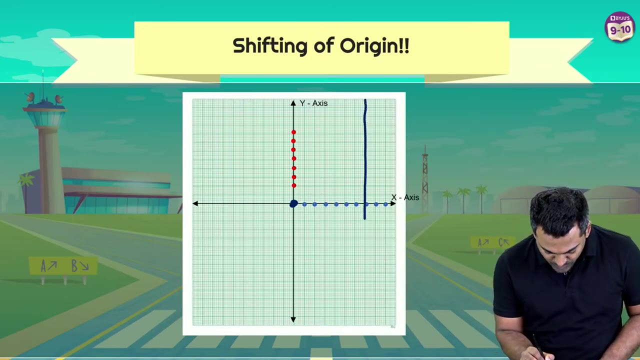 so if I want to shift the origin- shift the origin means what? shift the place from where you are comparing. okay, like, let's suppose I do this, this is the origin. now, right, I cut it off and I want to make this as the origin. it's suppose this becomes my y-axis and let's say, this becomes my x-axis. let's suppose, and this becomes: 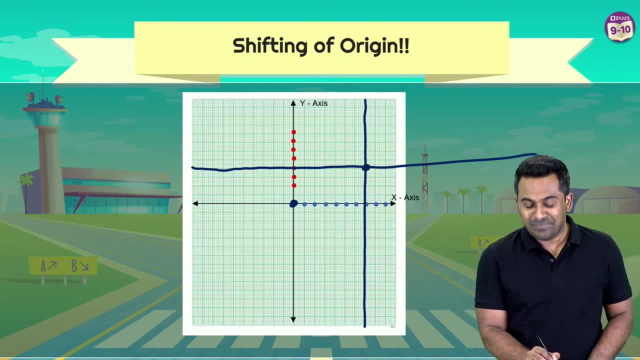 my origin, right? so this delhi airport location becomes what let's say now: this is your plus y, this is your plus x, this is your minus x and this is your minus y. let's say: this is the origin now. now, can you tell me the location of this point here, the delhi airport, with respect to the new? 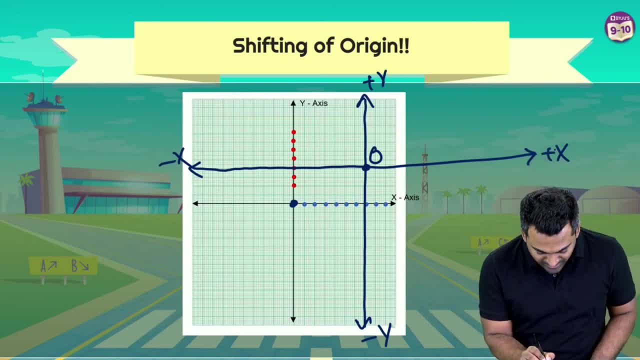 origin, which is the mumbai airport. now, yeah, so look, count, this is definitely in the third quadrant. so what will? the location x is one, two, three, four, five, six, seven right, so this is minus seven left. and then how much down? one, two, three, four down, so now the location becomes minus seven. 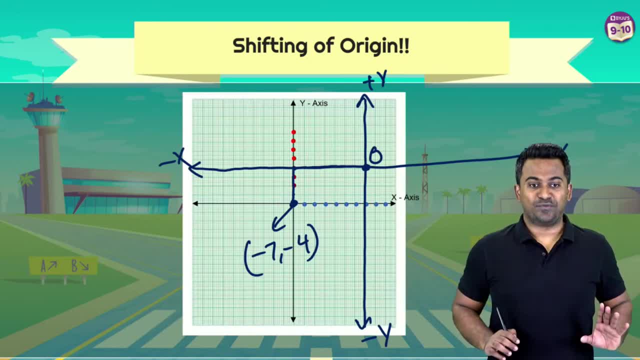 comma minus four. okay, so far, guys. that's it. right x positive, left x negative, right x, positive, left x negative, up y positive, down y negative. that's all. if you can remember this, you know the job for this session is done. we just wanted to make it a little interesting for you by introducing airplanes. the 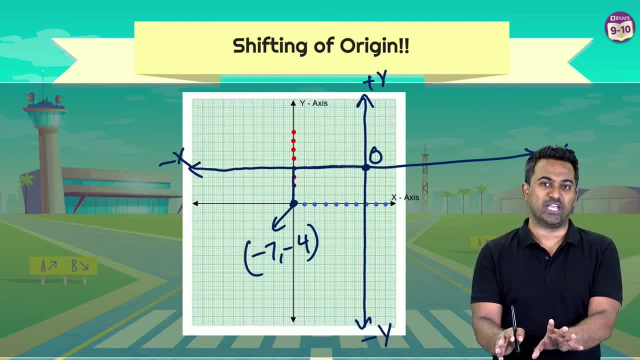 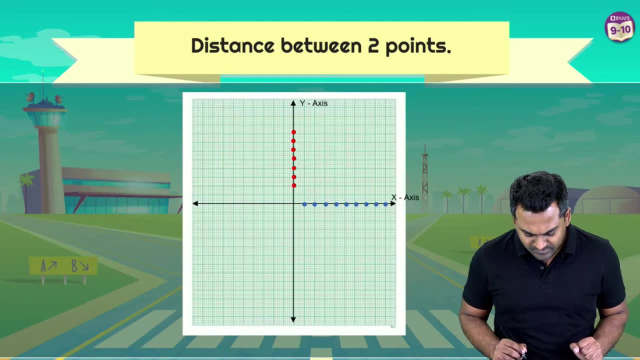 missing airplane, the story and all of that. but the heart and soul of this session today is to help you plot points on a coordinate plane and that's it, nothing much. all right, now i'm gonna play a little bit with you here. how many of you guys can tell me what is pythagoras theorem? i'm sure you. 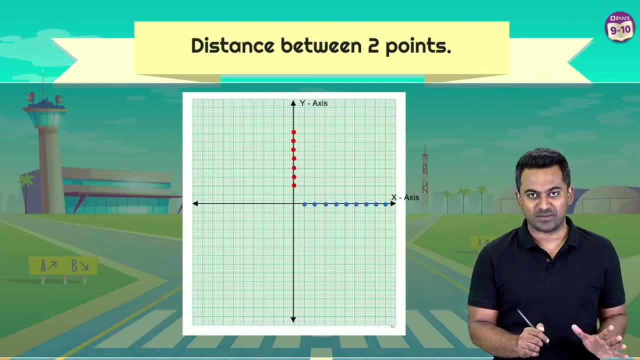 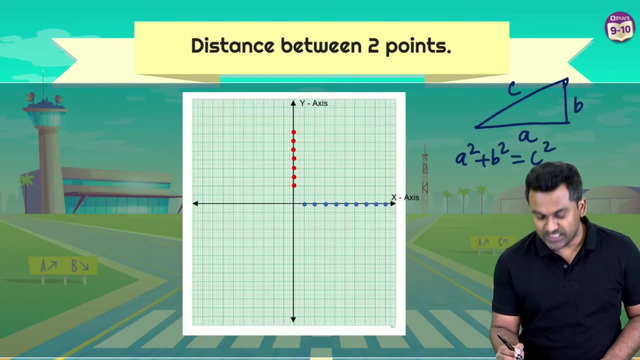 guys know the pythagoras theorem. we've just studied this in in the topic of number system, right? what is pythagoras theorem? what is the pythagoras theorem? if this is a, this is b, this is c, then according to the pythagoras theorem, a square plus b square is equal to c square, is it not? 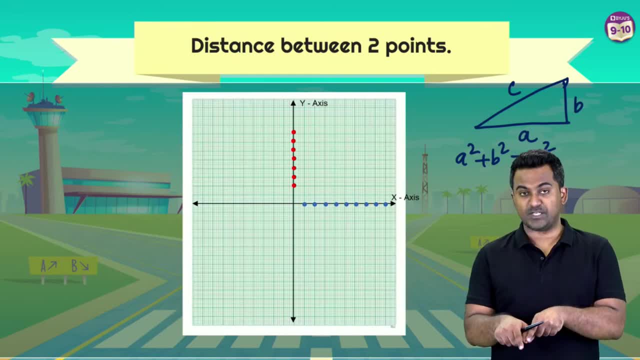 yes, according to pythagoras theorem, a square plus b square is equal to c square. now let's suppose this is the line. okay, and this is another line. let's suppose i'm joining this. let's say this is the delhi airport and let's say this point is the mumbai airport. 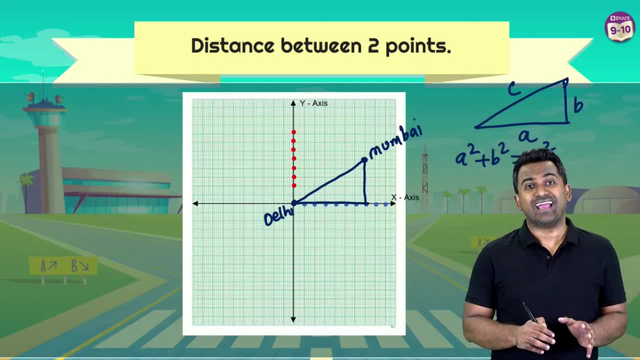 all right, you want to find the distance between the delhi airport and the mumbai airport. how are you going to do it? how are you going to do it? using the pythagoras theorem? right, because you will simply measure this: how much is this? one, two, three, four, five, six, seven, this distance is 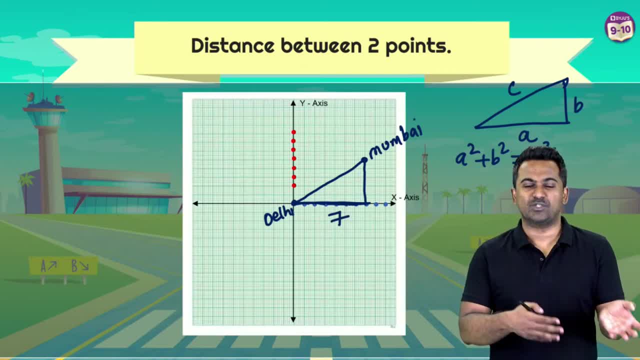 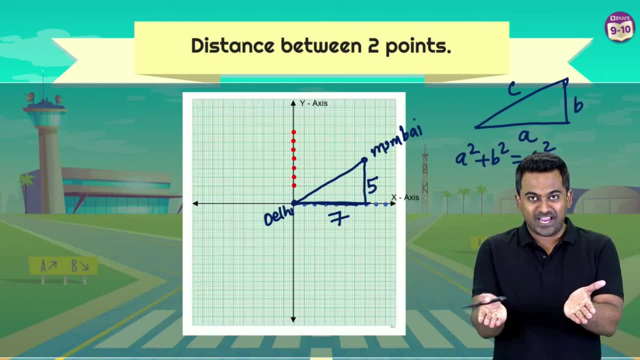 airport and mumbai airport now, because we know the horizontal distance is five and the sorry. the horizontal distance is seven and the vertical distance is five. so, using this idea, you can find the distance between the delhi airport and mumbai airport now because we know the horizontal distance. 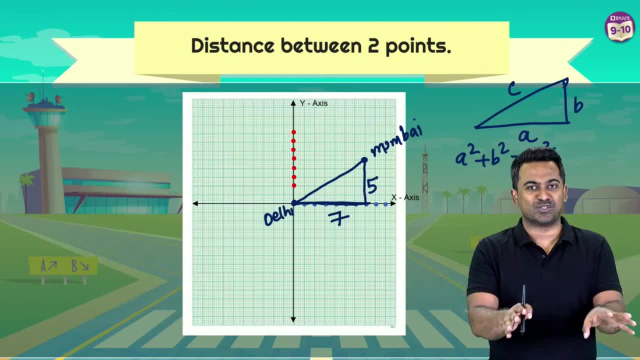 between the airports as well. there will be a formula as well, but for now you don't need to focus on formula. pythagoras theorem is enough. so this will be what seven square plus five square under root, which is going to be 49 plus 25 under root. if simplify, what do you get? 49, 25, how much? 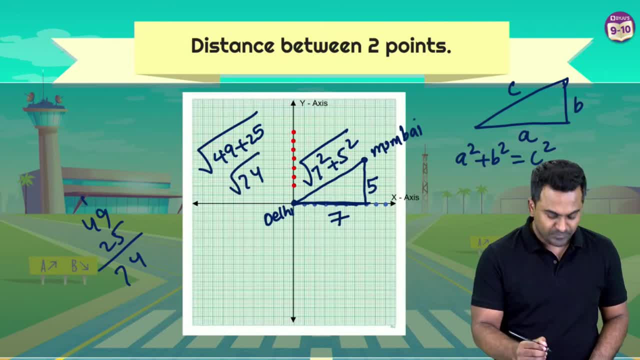 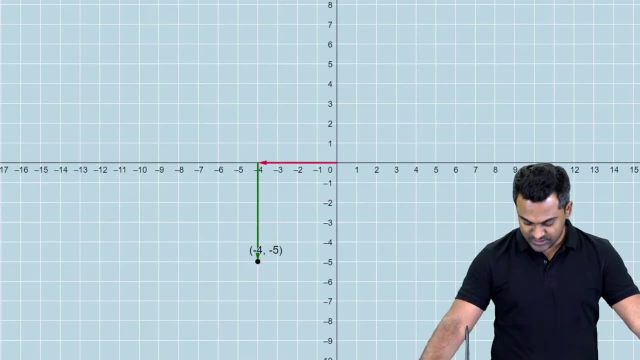 is that for 74, so square root of 74. so this is how you can also figure out distance between- uh, you know, one airport and the other. all right, so you've understood it. as i said, the heart and soul of this session today was this: plotting points on a coordinate plane. again one last. 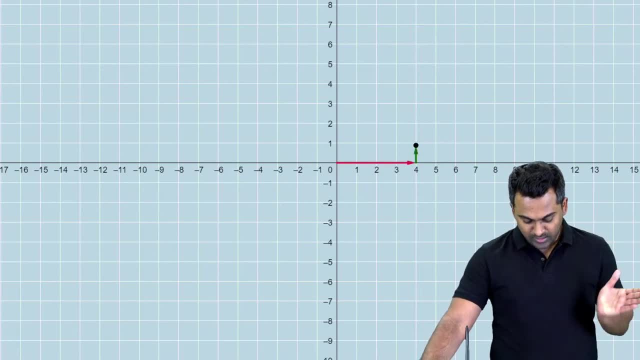 example, and then we'll call it off: okay, four comma eight. look right, four up eight. because why both positive? new example: zero comma minus eight. sorry, minus three. comma minus seven. x minus three, y minus seven. just remember the direction: minus one, comma minus nine, x minus one, y minus nine. 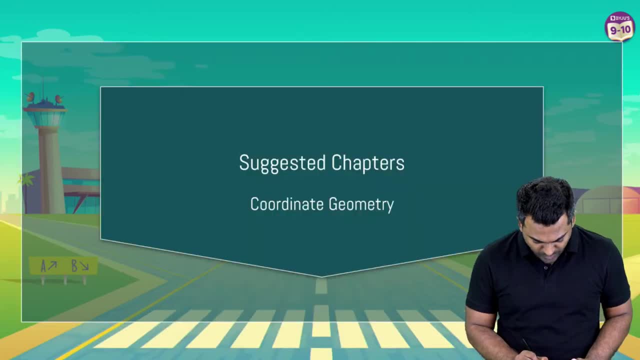 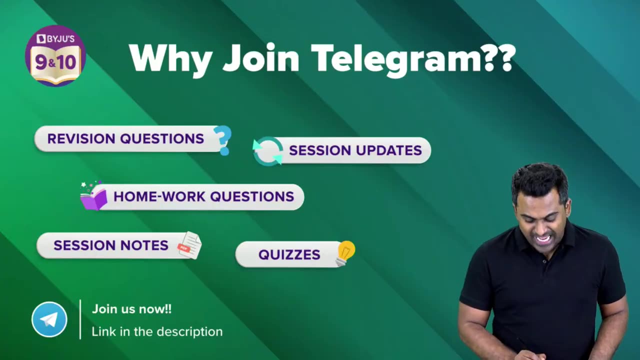 that's all come on. moving on now, as i said, this was the beginning of coordinate geometry and, uh, we've come to the end of the session. uh, the topic, the concept that you've covered is what? how to plot points on a coordinate plane. as simple as that. again, i've got to remind you students who have joined in the 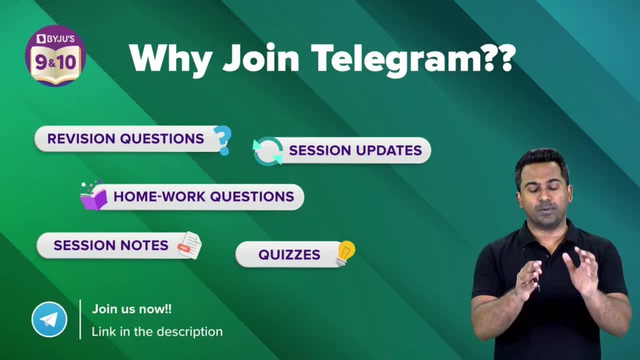 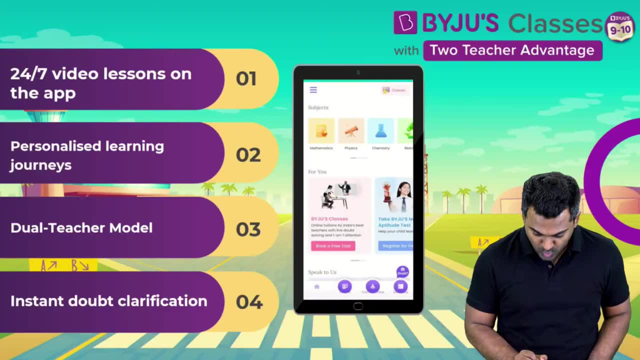 middle of the session. please don't miss out. there'll be a link to this uh telegram channel in the description of the video. please make sure you join this channel, especially for the session notes. and lastly, the by juice two teacher advantage: 24: 7 video lessons would. 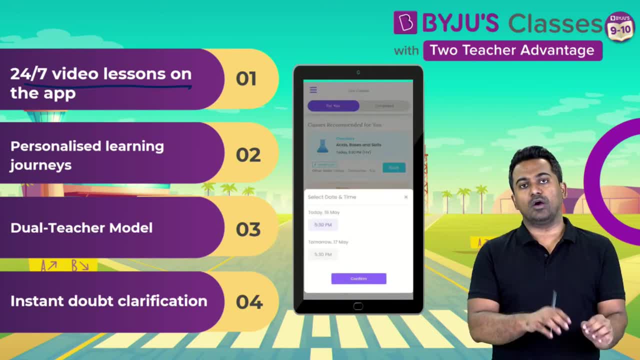 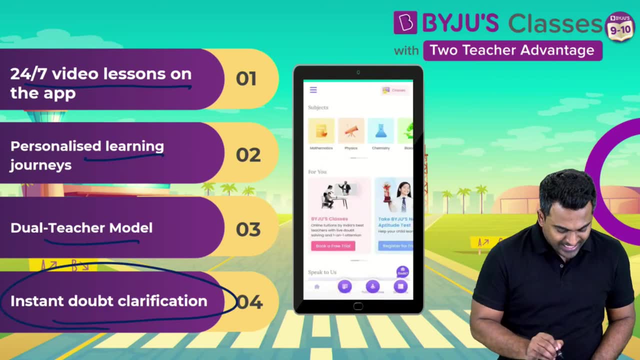 be there on the app. tremendous amount of, of, you know, uh, conceptual clarity, uh, the kind of that we've seen so far- personalized learning journeys, then the tour teacher model, and then you have the instant doubt clarification and uh, last, you know, if you've liked it, hit the. 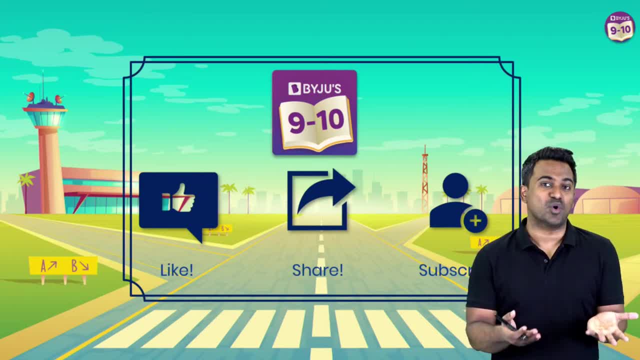 like button, share it with your friends and if new students have joined us, please make sure you subscribe. all right, so have you understood it? yeah, i hope you guys have understood how to plot points on a coordinate plane- as simple as that, right? so please make sure you practice this out, and i'm going to see.